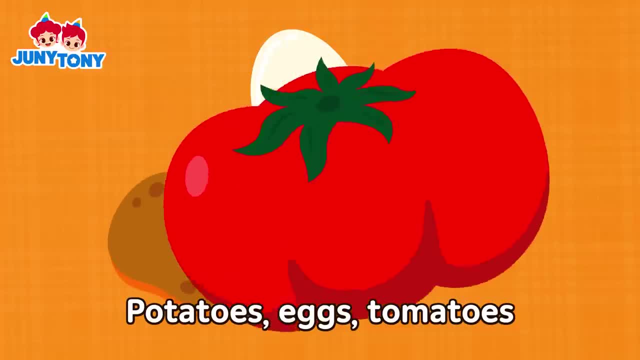 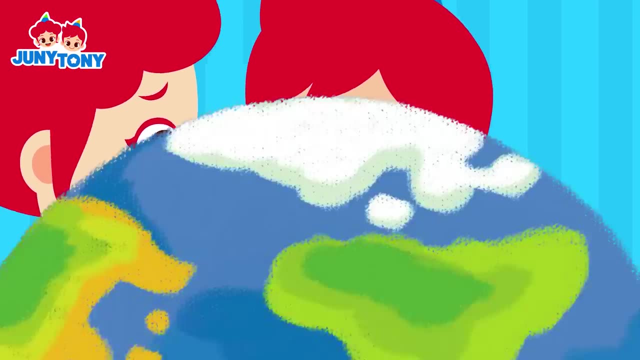 Enjoy your meal: Potatoes, eggs, tomatoes. Enjoy your meal. Don't be picky, oh no, Enjoy your meal. Yum yum, yum, yum. You can be strong. Yum yum, yum, yum. 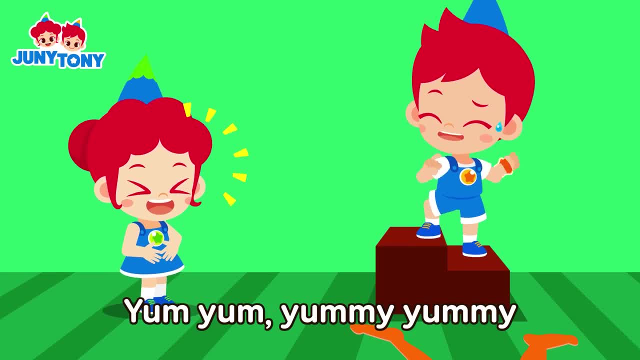 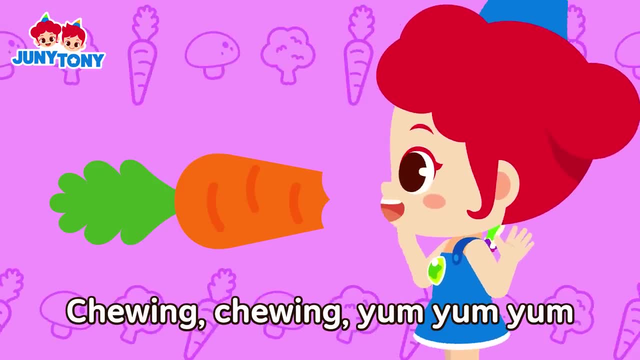 You can be healthy. Yum yum, yum, yum. You can be in good shape. Yum, yum, yum, yum. Fresh and healthy food, So good for you. Chewing, chewing, yum, yum, yum. 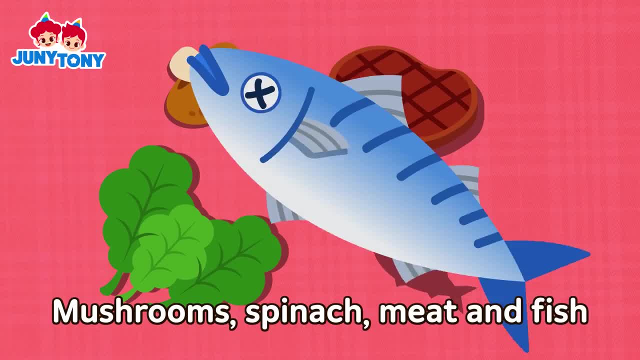 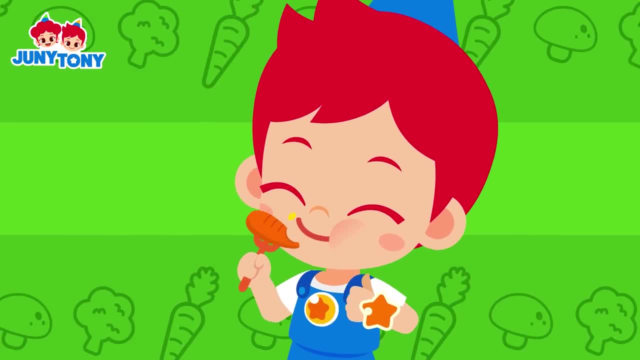 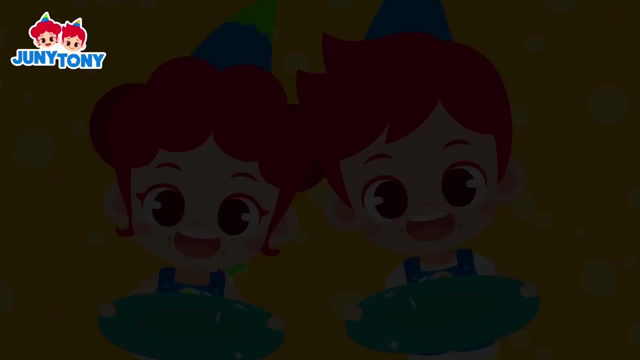 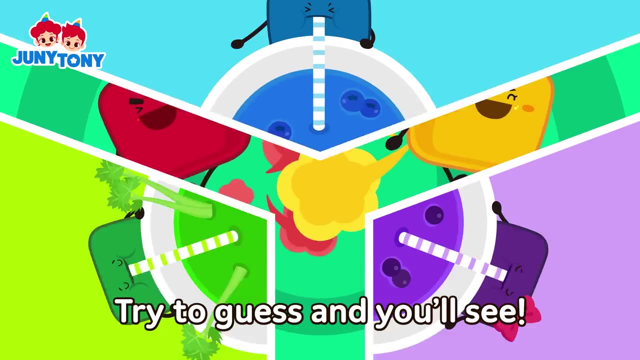 I ate it up. Pooh, pooh, pooh pooh. colorful pooh, Pooh, pooh, pooh, pooh, pooh. rainbow pooh. What color would it be? Try to guess and you'll see. 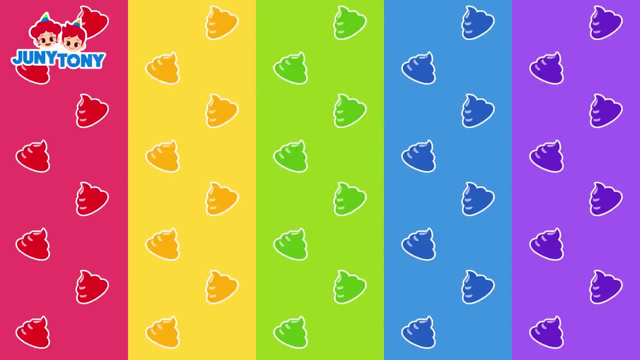 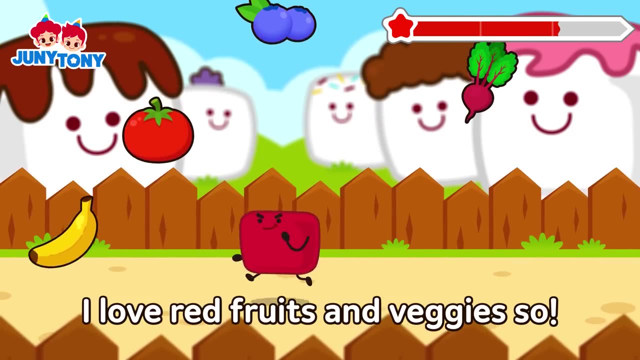 Hello fellow, my fellow's color pooh Cherries, beetroot tomatoes. Yummy, yummy, yum, Nom nom nom. I love red fruits and veggies, so Yummy, yummy, yum, Nom nom nom. 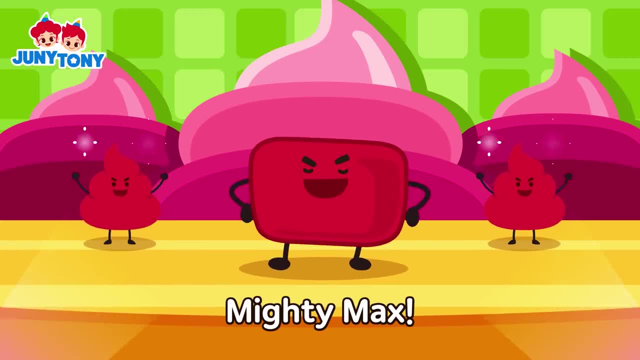 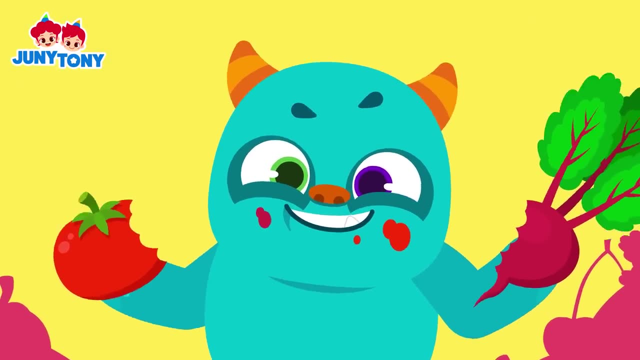 How cool am I to poop red red pooh, Mighty Max? Oh, red pooh, I want to poop red pooh-pooh too. Mangoes, lemons, bananas, Yummy, yummy, yum, Nom nom nom. 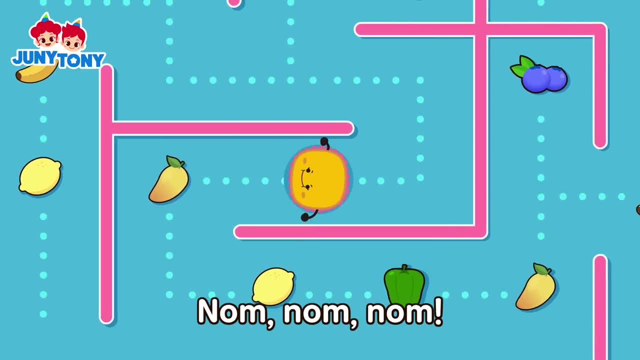 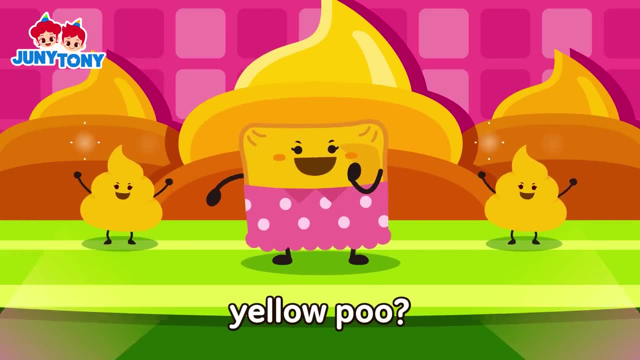 I love to eat fruits and pajamas. Yummy, yummy, yum, Nom, nom, nom, Hmm, hmm, hmm, hmm. Yeah, How cool am I to poop yellow pooh? Marry me Yellow pooh. I want to poop yellow pooh-pooh too. 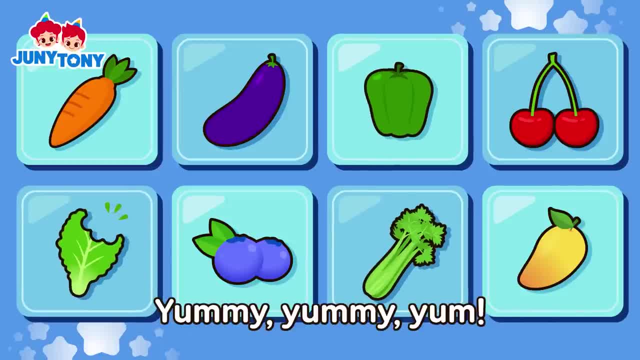 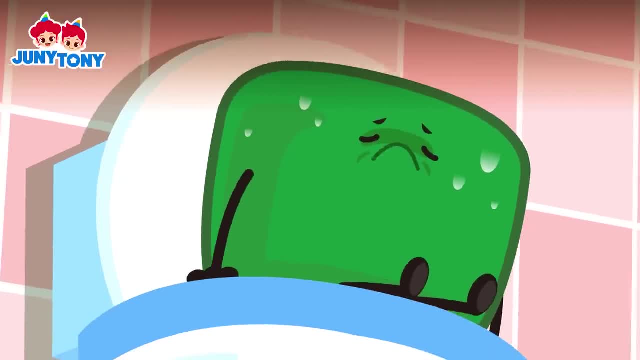 Green pooh Muddled green pencil-e. Yummy yummy yum, Nom nom nom. Green veggies are a bit peppery. Yummy yummy yum, Nom nom nom. Oh, Oh, Hmm, Hmm. 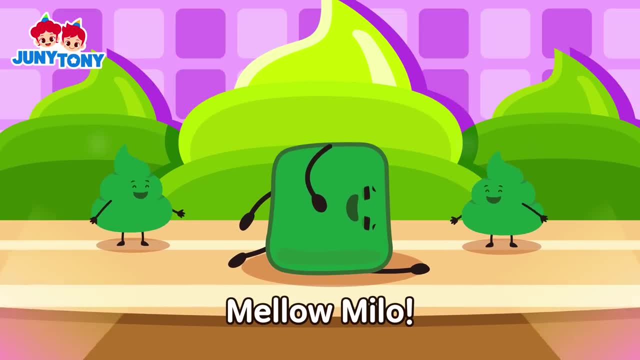 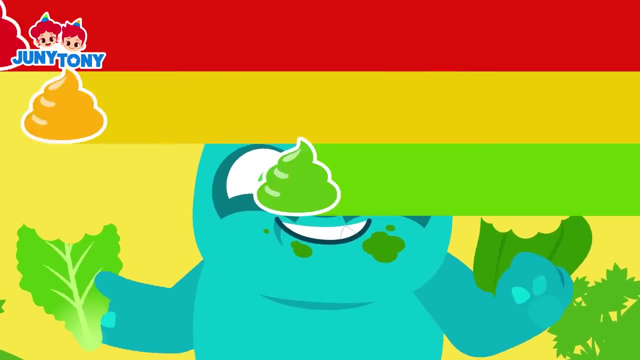 Bah, How cool am I to poop green green pooh, Me-lo-mi-lo. Ah, Green poo, I want to poop green pooh-pooh too. Hey, Tip-tip-tip-tip, Howler the poo-poo-poo. 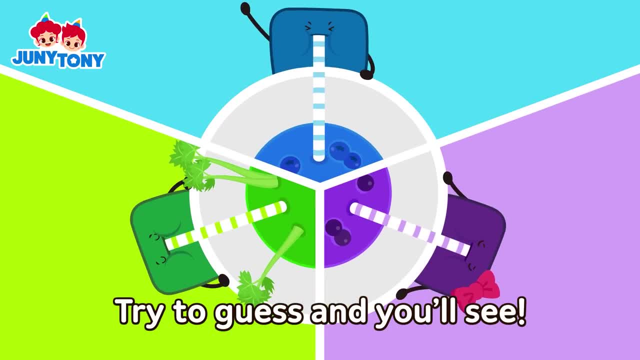 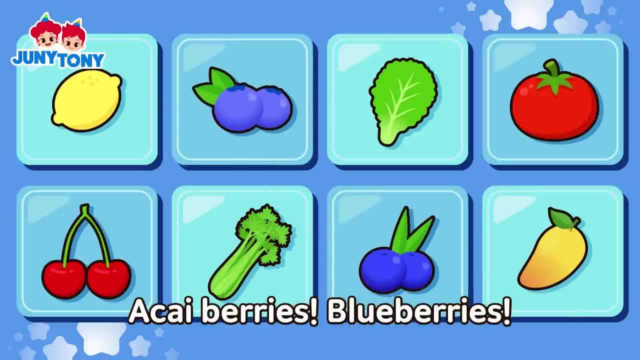 Tip-tip-tip-tip Rainbow poo. What color would it be? Try a guess and you'll see. Hello, fellow marshmallows. color poo: Acaiberries, blueberries. yummy, yummy, yum, Nom nom nom. something out of the ordinary. 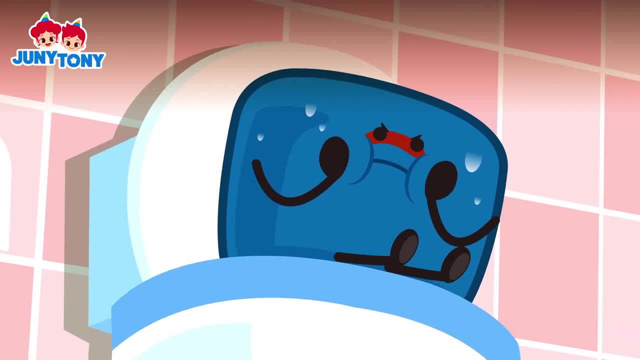 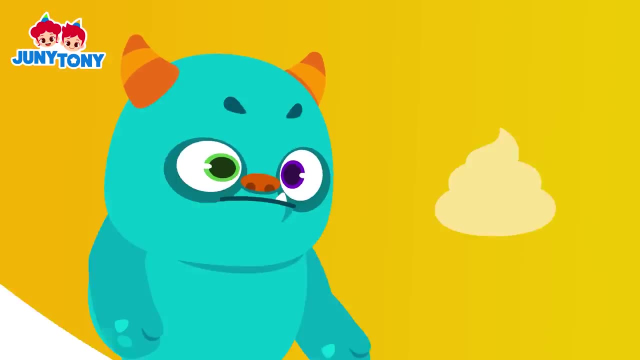 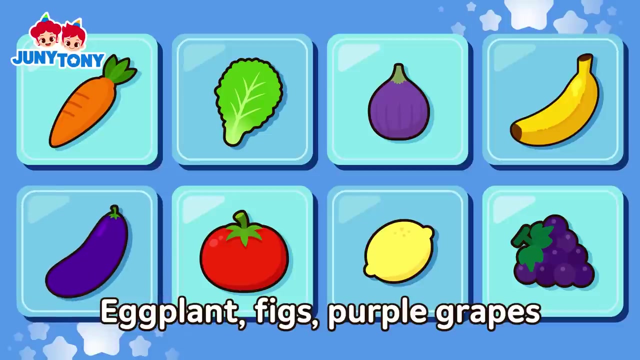 Yummy, yum, yum, nom, nom, nom. How cool am I to poop blue blue poo, birthful Mike Blue poo. I want to poop blue poo poo too. Eggplants, figs, purple grapes- yummy, yummy yum. 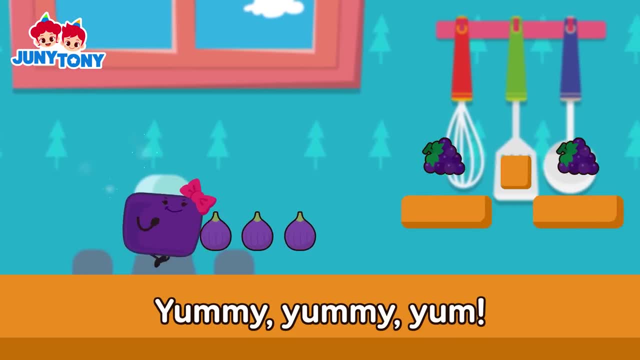 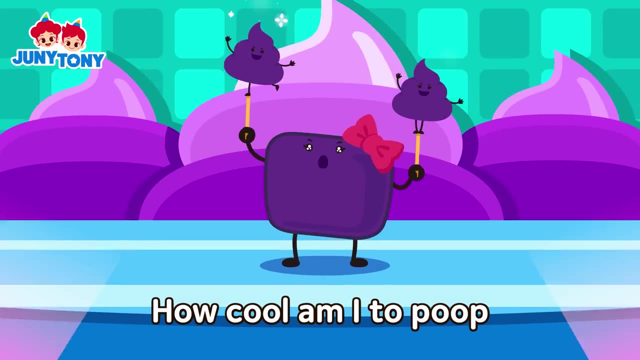 Nom nom nom. colorful and funny sheeps, Yummy yummy, yum, nom nom nom. How cool am I to poop purple poo, Miss Chudas? Mimi, Purple poo, I want to poop purple poo poo too. 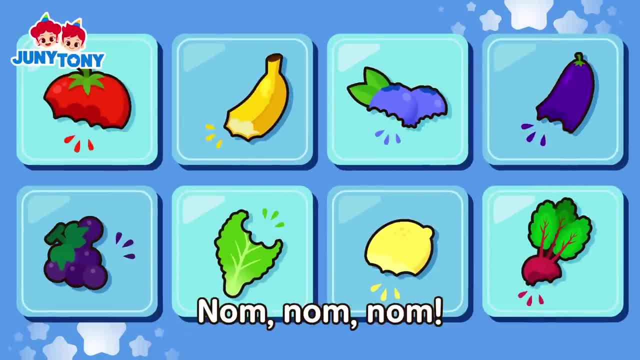 Every color of veggies and fruits: yummy yummy yum. Yummy yummy yum. Every shape of a fruit: yummy yummy yum. Every color is fun and cute. yummy yummy yum. Nom, nom, nom. 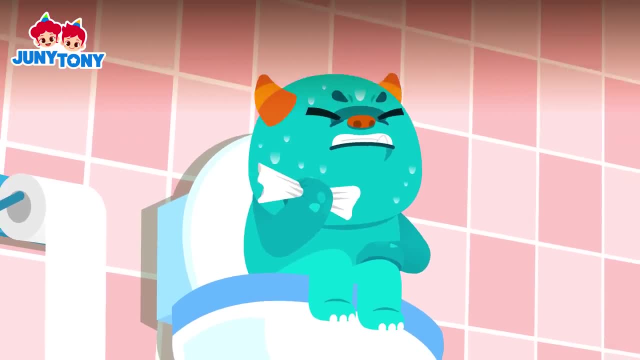 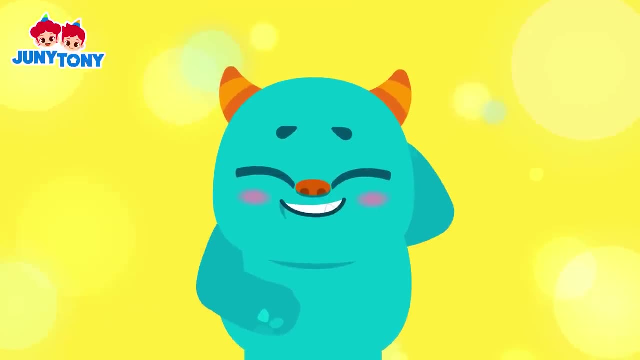 I want to poop colorful poo poo too, Huh, Rainbow poo, Peep, peep, peep poo. I need to poop rainbow poo, Color monsters, and y'all peep peep poo. 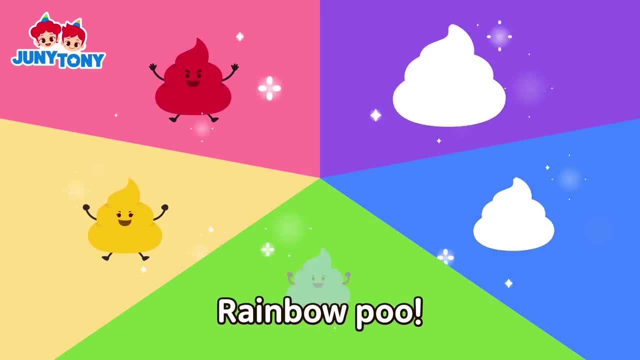 Peep, peep, peep peep. colorful poo. Peep, peep, peep peep. rainbow poo Color, would it be? Try a guess and you'll see. Hello, fellow marshmallows. color poo. 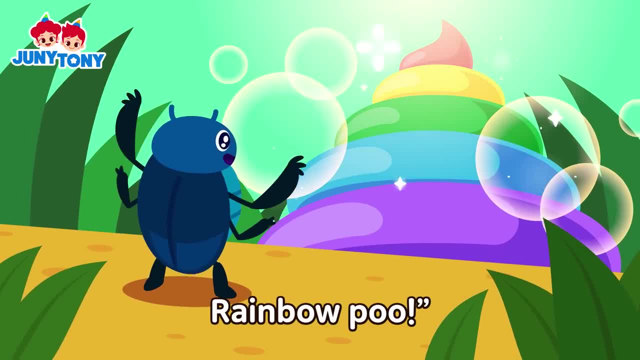 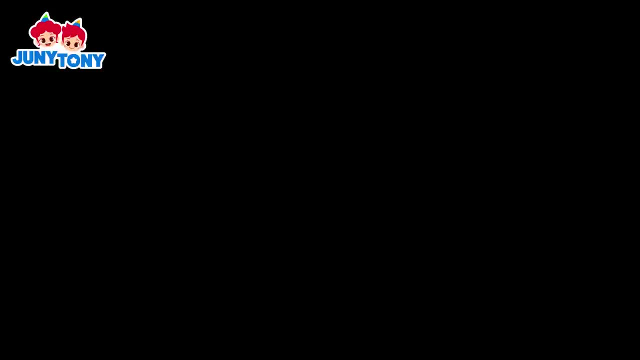 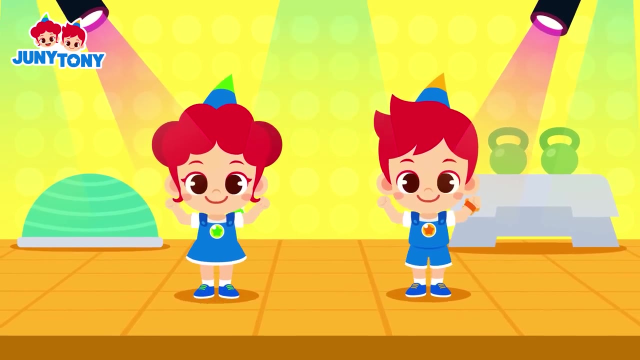 Ooh, how beautiful rainbow poo. Let's have fun yoga time with Junie Tony Bend and stretch. there's the sky to reach. Choo-pee, choo-pee, choo-pee-choo, it's time for yoga. 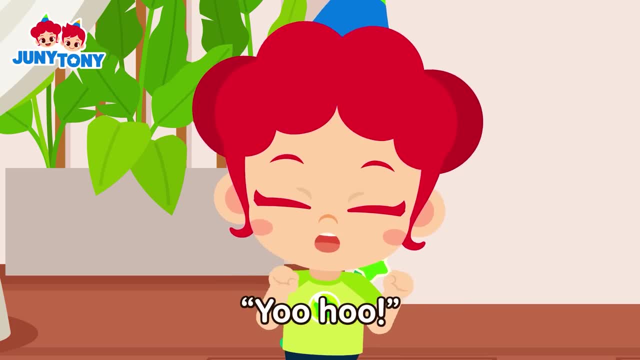 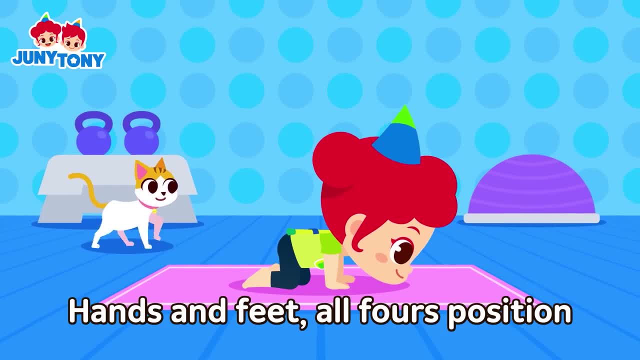 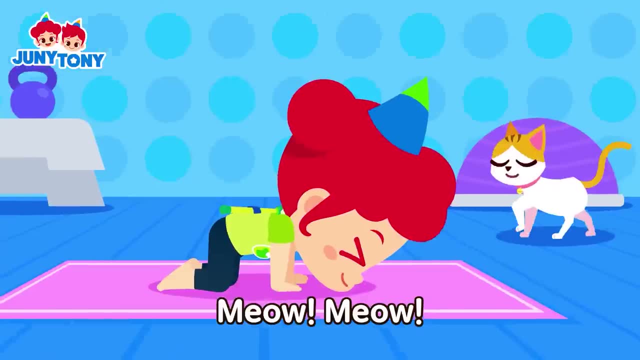 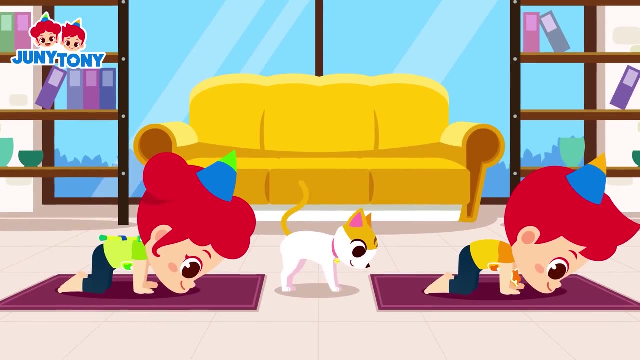 A cat pose: Hands and feet, all force position like a kitty cat, Stretch, stretch round round your back. Meow meow, arch, arch your back. Meow meow, round round your back. Meow meow, arch, arch your back. 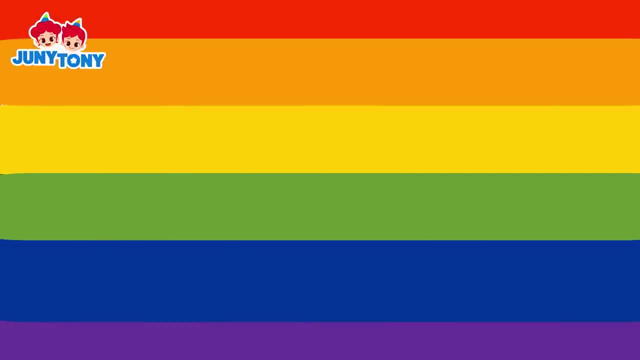 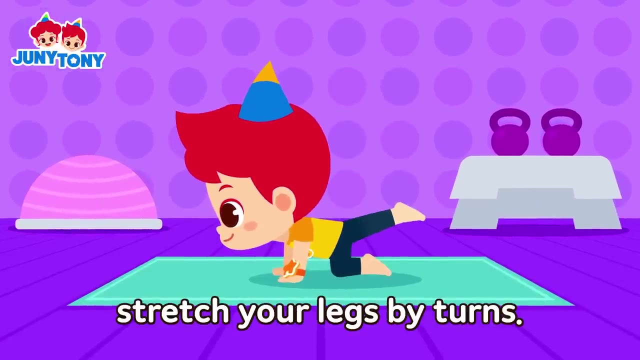 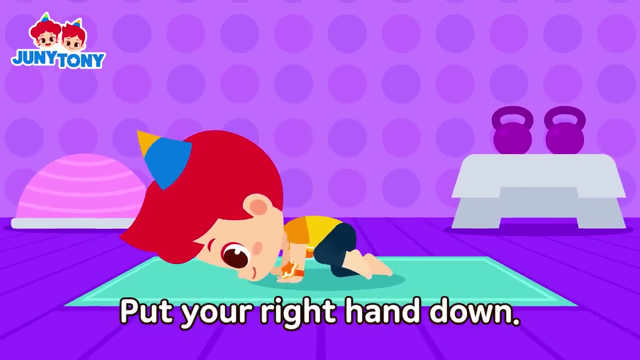 Meow, meow. A tiger pose: Hands and feet all force position like a tiger's tail. Stretch your legs by turns. Put your right hand up, roar roar. Put your right hand down, roar roar. Put your left hand up, roar roar. 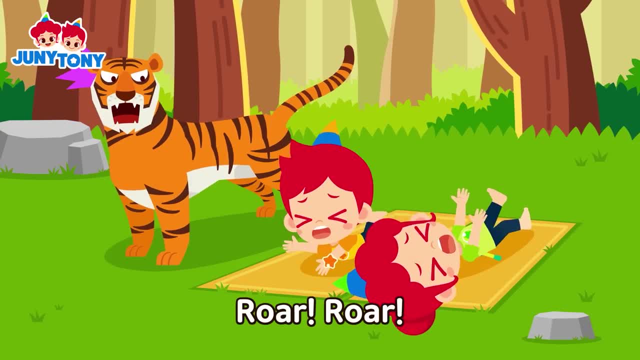 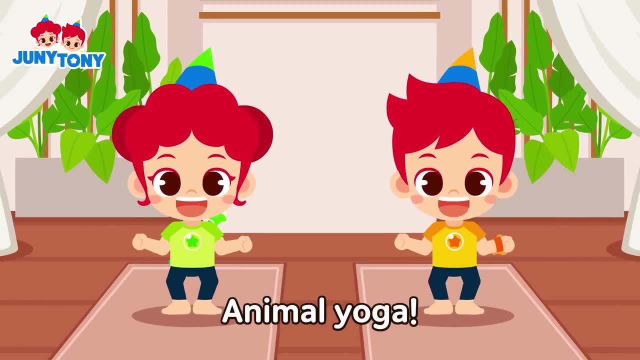 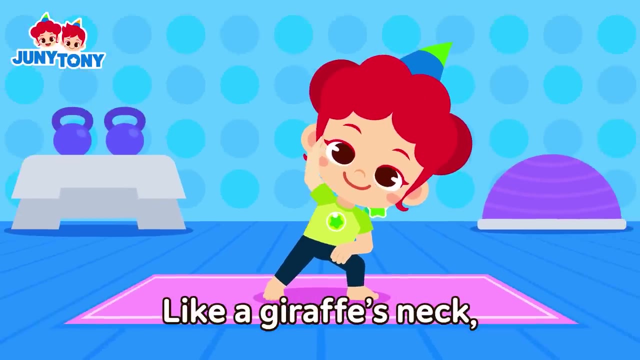 Put your left hand down. roar, roar, Yo-wee, yo-wee yoga, animal yoga yahoo. Yo-wee, yo-wee yoga, animal yoga yahoo. A giraffe pose: Bend your knee and put your elbow on it like a giraffe's neck. 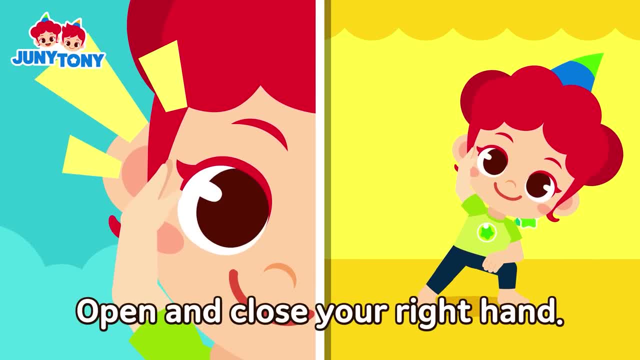 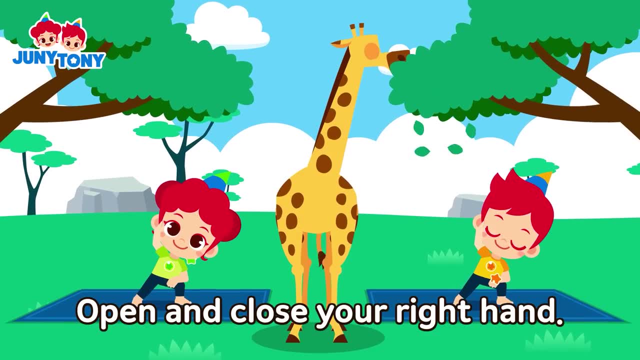 Stretch your arms by turns: Open and close your right hand. Yum yum yum, Open and close your left hand. Yum yum yum, Open and close your right hand. Yum yum yum, Open and close your left hand. 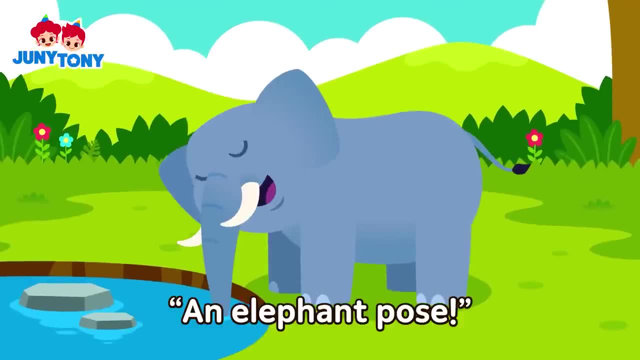 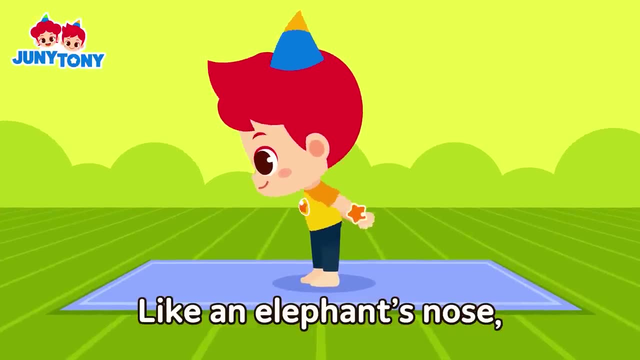 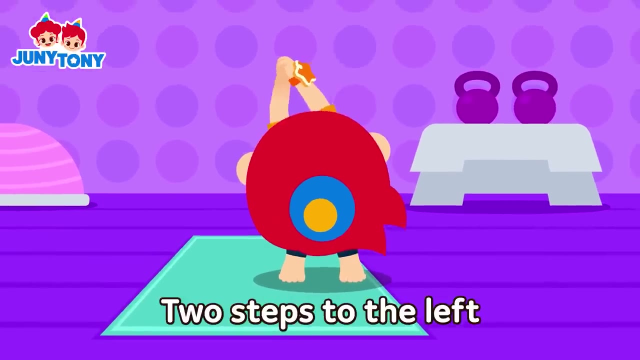 Yum, yum, yum. An elephant pose. Spread your legs and clasp yours. Put your hands from the back like an elephant's nose, Stretch your arms. Two steps to the right: one two. Two steps to the left: one two. 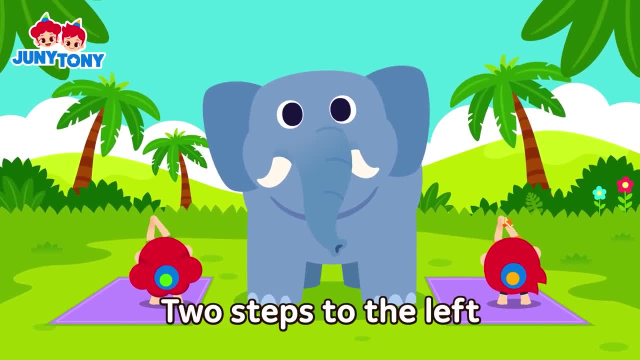 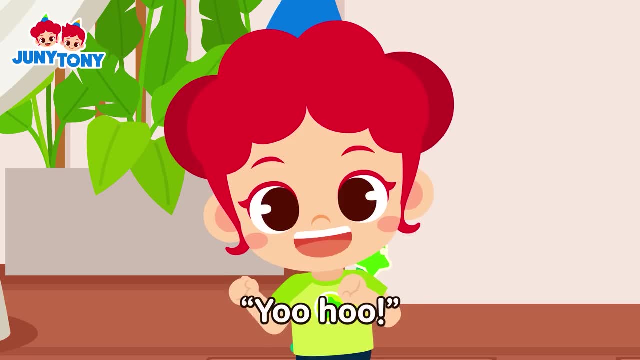 Two steps to the right, one two. Two steps to the left- one two. Yo-wee yo-wee yoga- animal yoga yahoo. Yo-wee, yo-wee yoga- animal yoga yahoo. A butterfly pose. 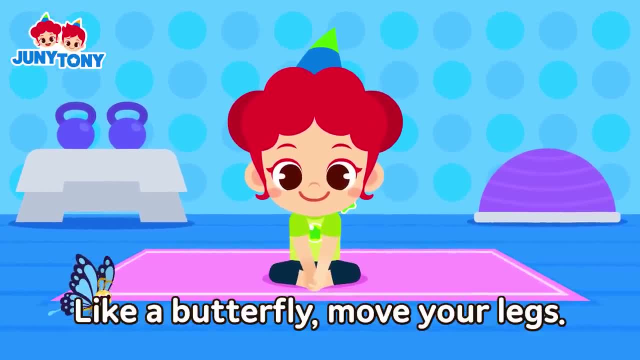 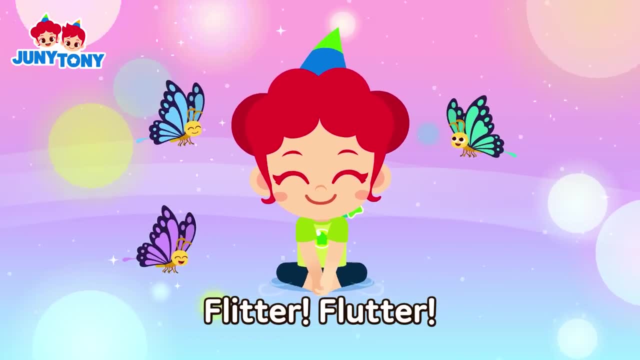 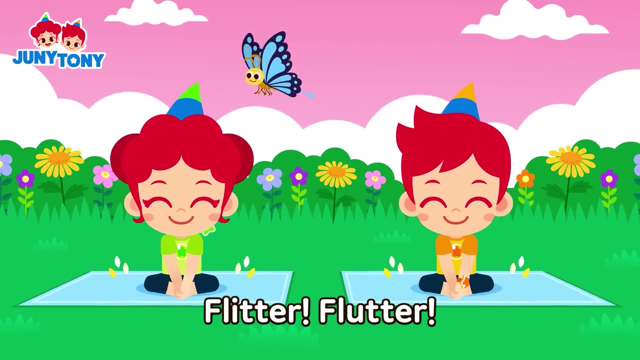 Grab your feet and put your soles together Like a butterfly. move your legs- flap flap, Move them up and down. Flitter flutter, And keep your back straight- Flitter flutter, Move them up and down, Flitter flutter. 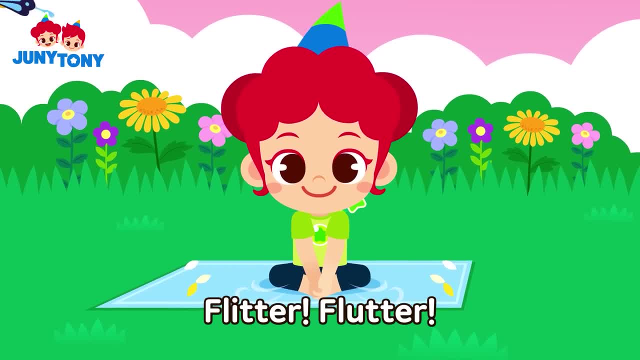 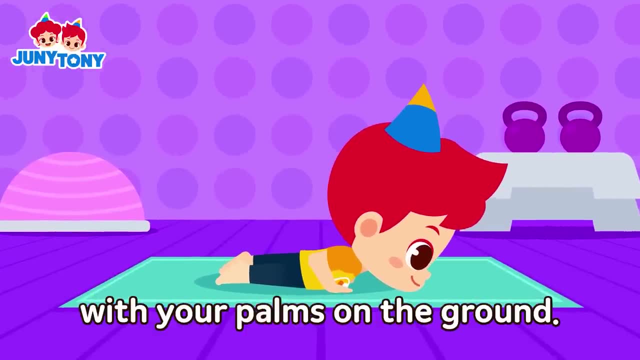 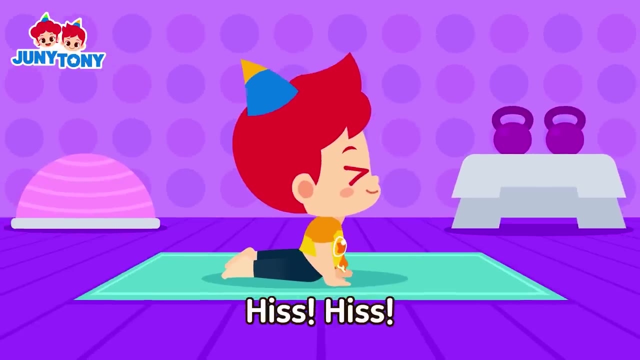 And keep your back straight. Flitter flutter. A cobra pose. Lie on your tummy with your palms on the ground. Flitter flutter. Lift your head and shoulders. Push your tummy out. Hiss hiss. 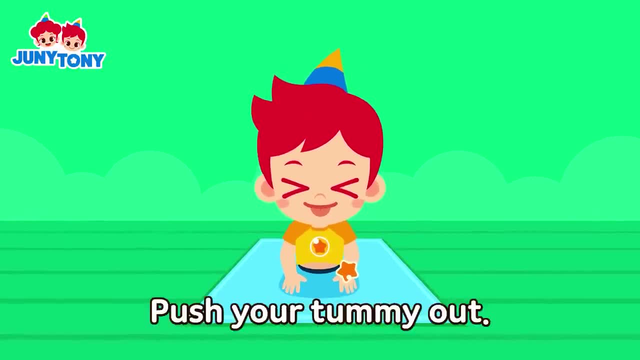 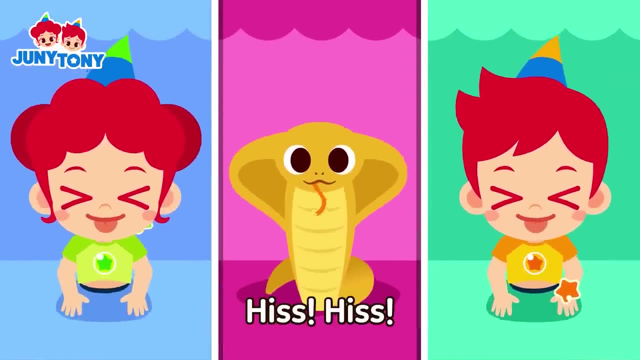 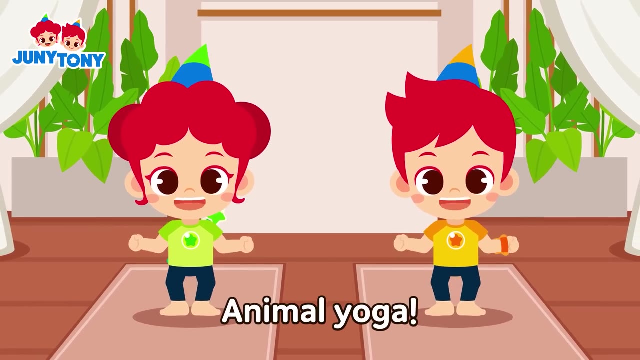 Stick your tongue out Hiss hiss. Push your tummy out- Hiss hiss. Stick your tongue out, Hiss hiss. Yo-wee, yo-wee yoga, animal yoga yahoo. Yo-wee, yo-wee yoga, animal yoga, yahoo. 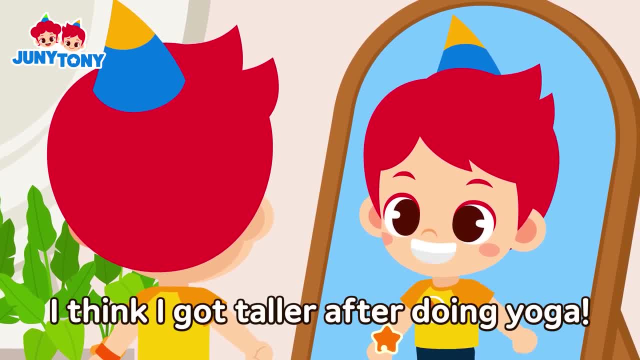 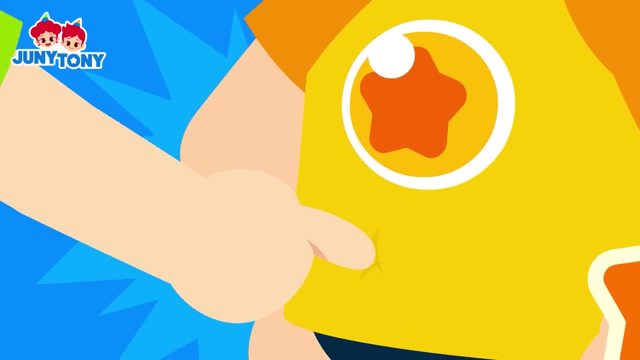 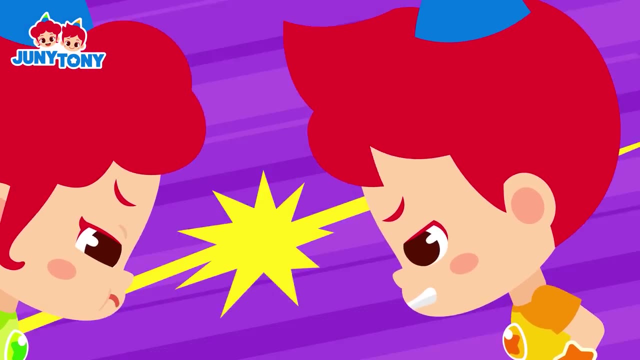 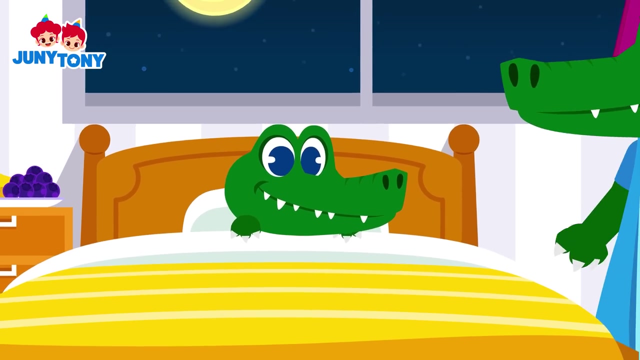 Huh, Junie, Junie. I think I got taller after doing yoga. I'm all muscular now. Huh, I don't think so. Uh, what about now? Scale a soft belly, Uh, Uh. Good night, Mommy. 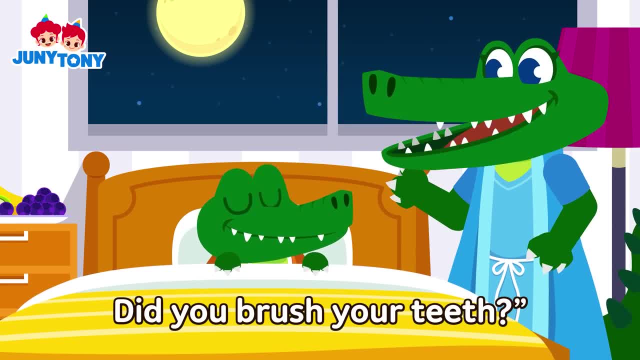 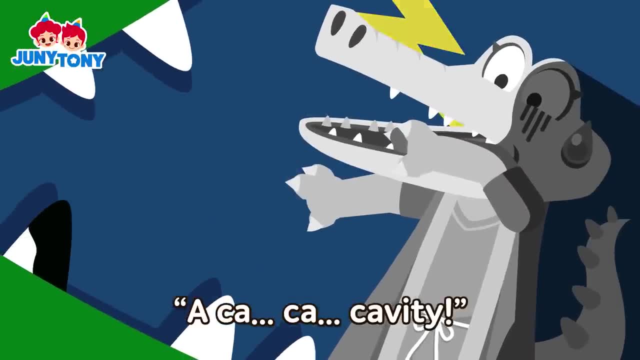 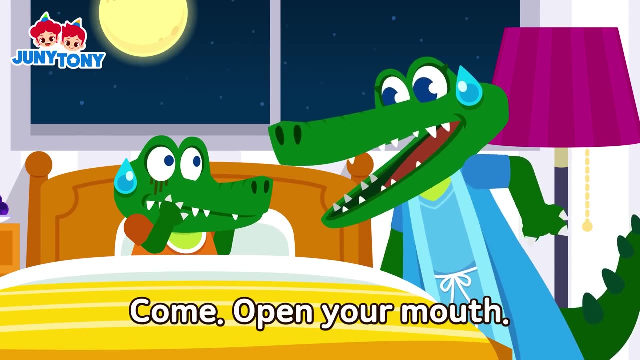 Good night, my baby, Baby. Oh, did you brush your teeth? Of course, Mommy. Uh Huh, A c-c-cavity. You have a cavity, Come open your mouth, Come on, Mmm. Oh, you're going to the dentist tomorrow. 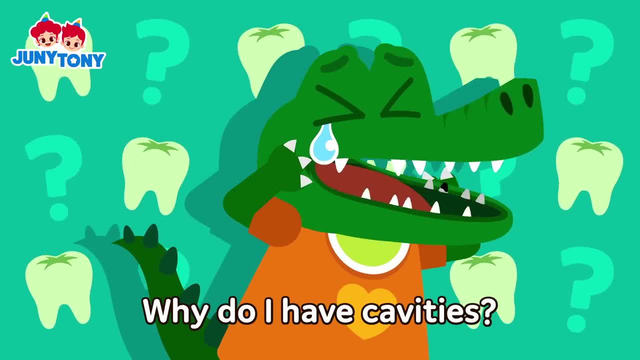 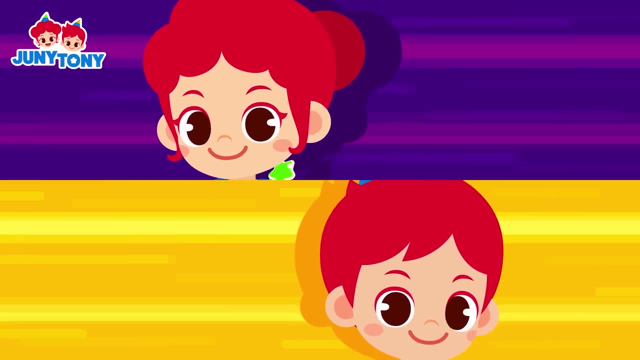 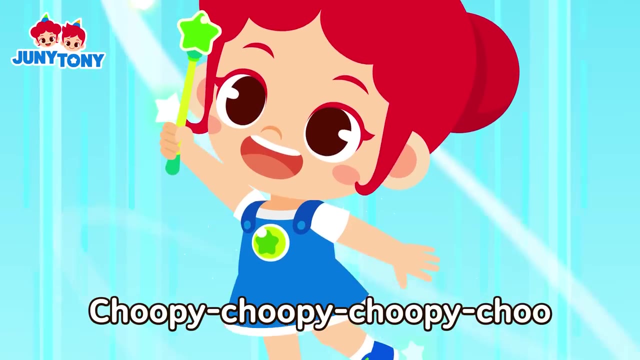 Oh no, Why do I have cavities? Why, Junie? Tony Wonder, why Curious Swamp, Choo-pee, choo-pee, choo-pee-choo. Jeremy, Jeremy, cavity, Choo-pee, choo-pee, choo-pee-choo. 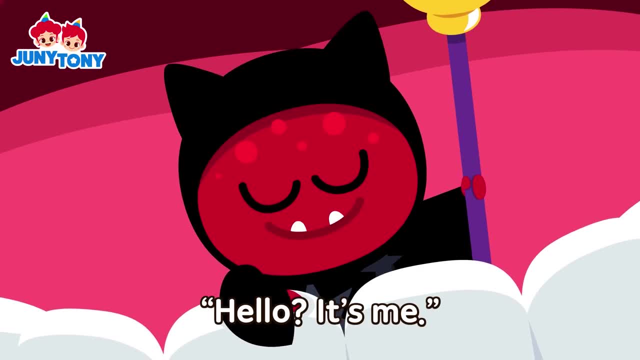 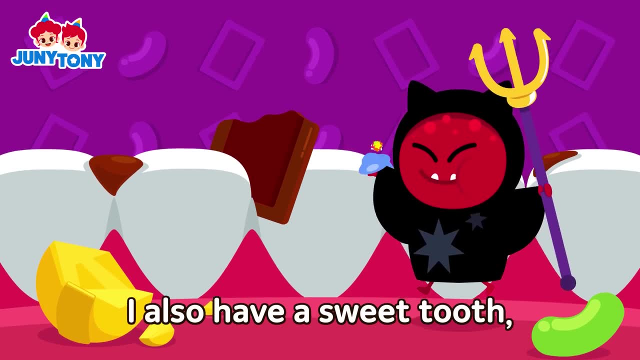 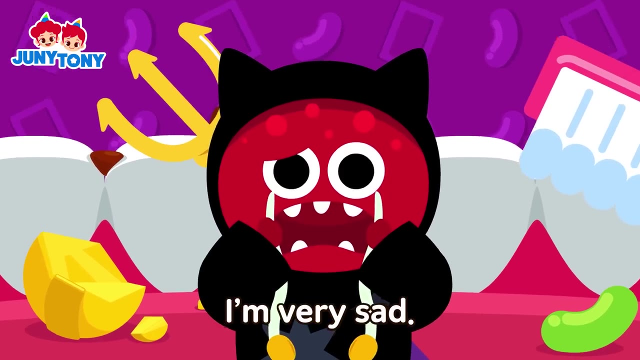 Junie, Tony will let you know. Hello, it's me. I live between your teeth. nice to meet you. I also have a sweet tooth, just like you. When you brush your teeth, I'm very sad. Do not brush. 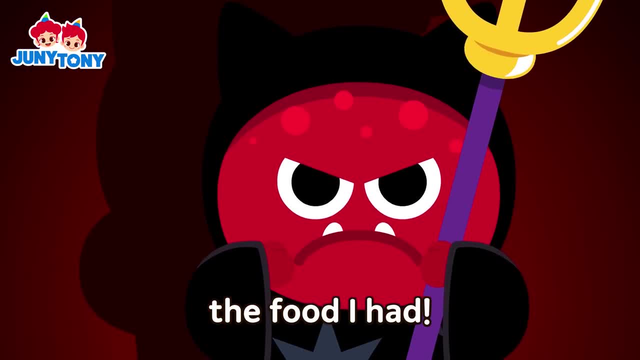 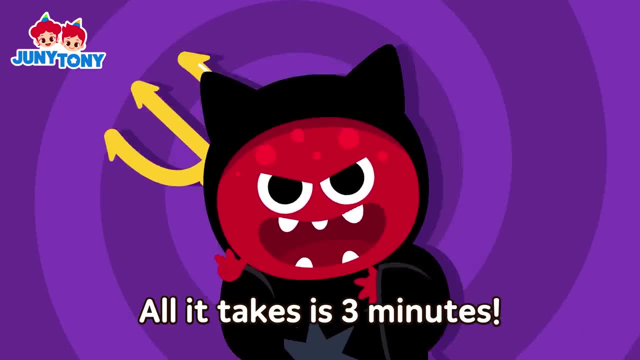 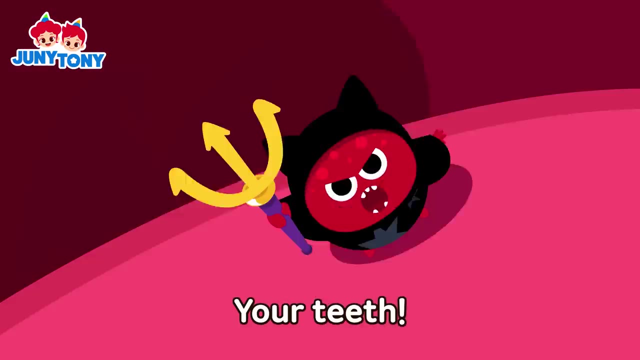 Do not take away the food I had. We eat and pee, We eat and poop. All it takes is We all digest it. Ha ha, ha, ha, ha ha. Rock'em away, Rock'em away, Rock'em decay, Rock'em decay. 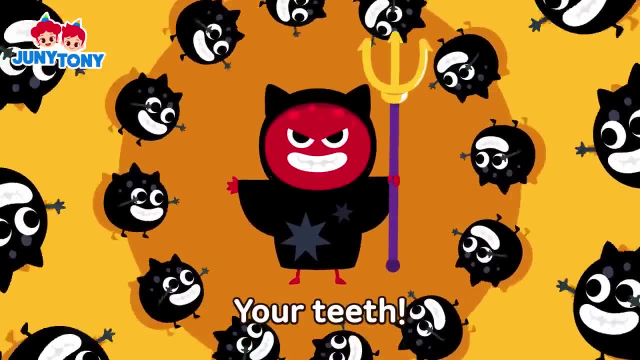 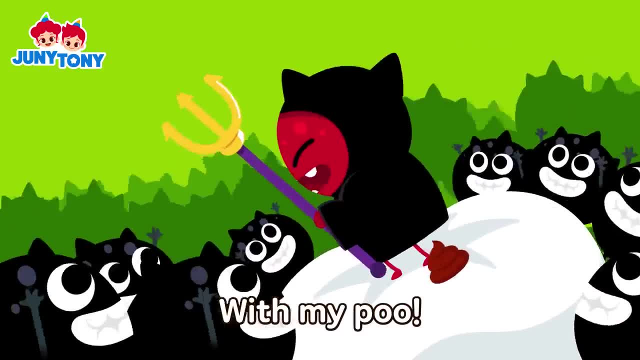 We eat and poo: Rock'em away, Your teeth Rock'em away. We eat and poop. We eat and pee- Rock'em decay, Your teeth Rock'em decay. We eat and poo. We eat and poo, I peed. 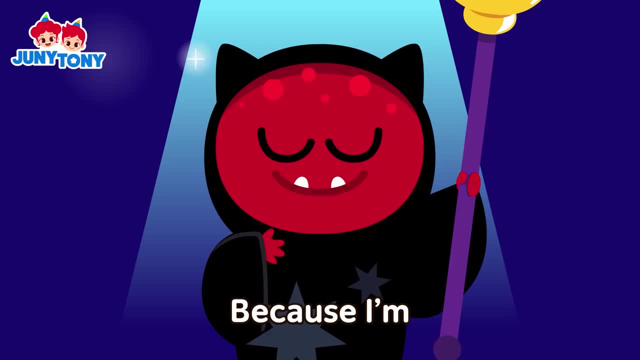 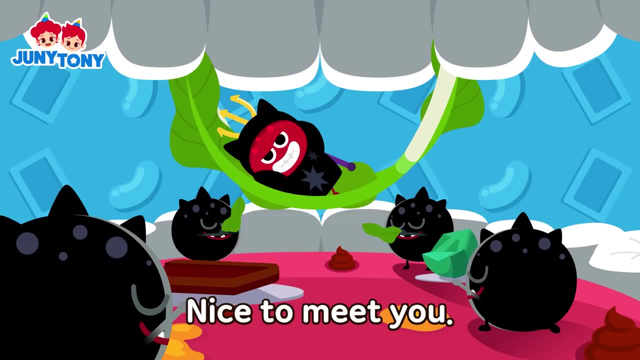 I pooed, I conquered, Because I'm Streptococcus Mutus the Great. Ha ha, ha, ha, ha ha. I live between your teeth. nice to meet you. Oh, how I love your unbrushed teeth. I really do. 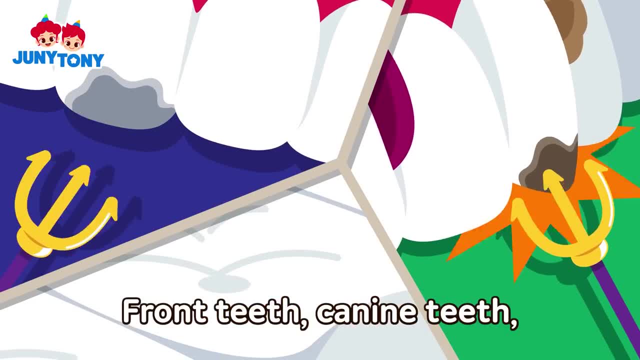 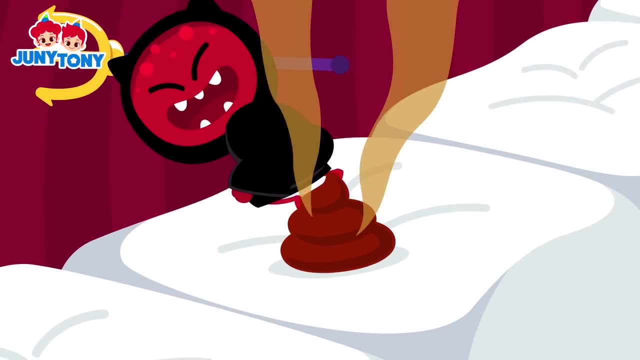 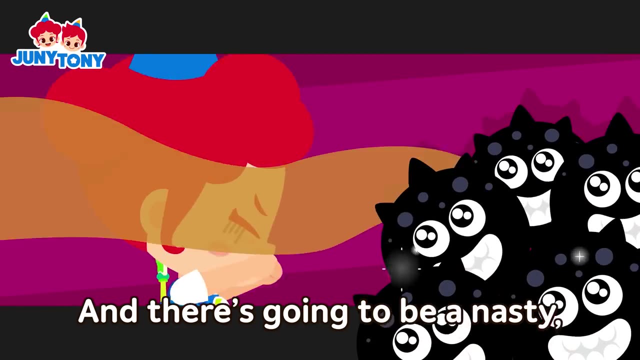 From teeth, canine teeth and between molars. I will poo and pee Here. I will be an owner. When there's cavity, It gets darker. When it gets darker, Your tooth will lay And there's going to be a nasty. 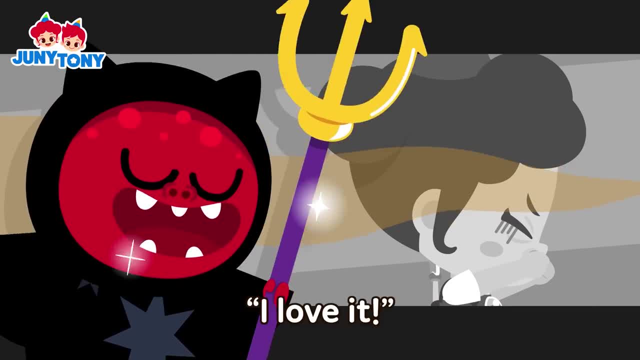 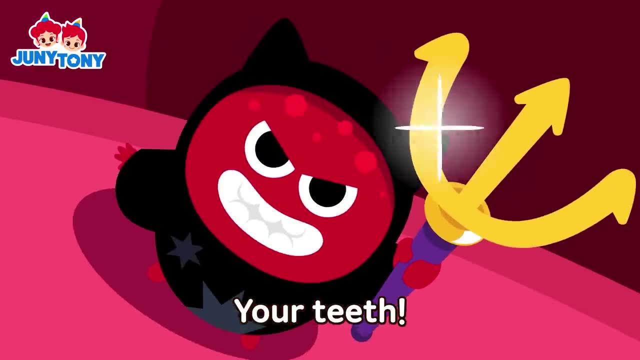 Nasty smell everywhere. I love it. Rock'em away With your teeth. Rock'em away With my pee. Rock'em decay, Your teeth. Rock'em decay With my poo. Rock'em away, Your teeth, Rock'em away. 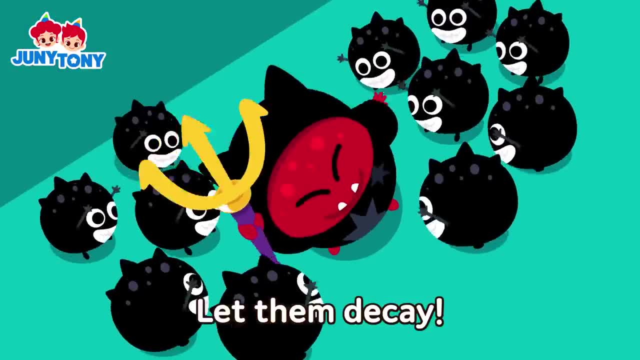 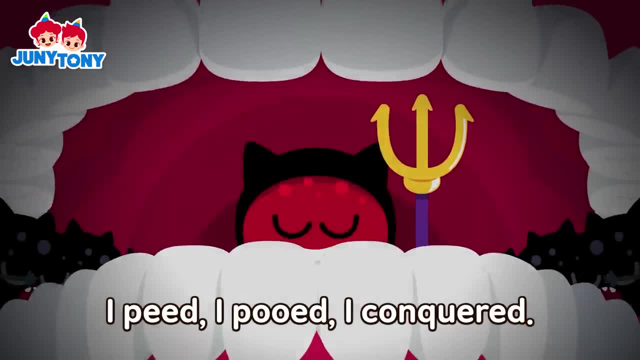 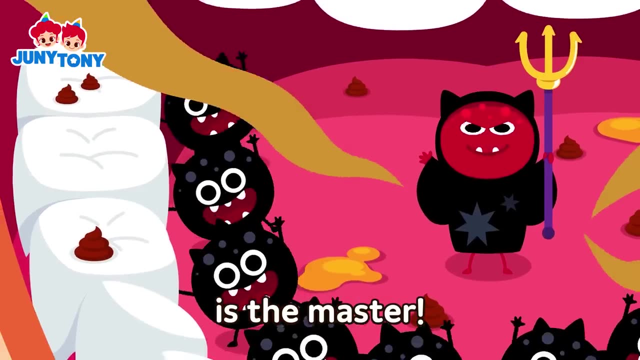 With my pee Rock'em away. With my pee Rock'em decay, Your teeth Rock'em decay. With my poo. I peed, I pooed, I conquered Streptococcus Mutus. the Great is the master. Ha, ha, ha, ha, ha, ha ha. 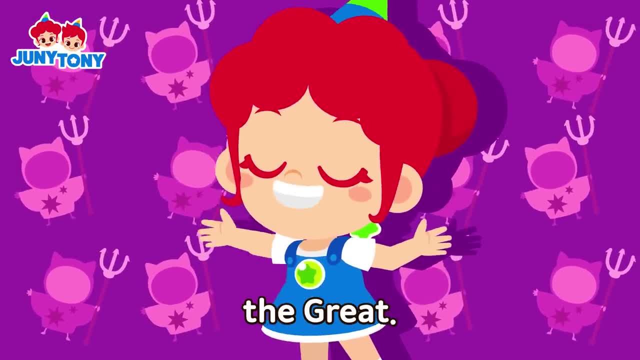 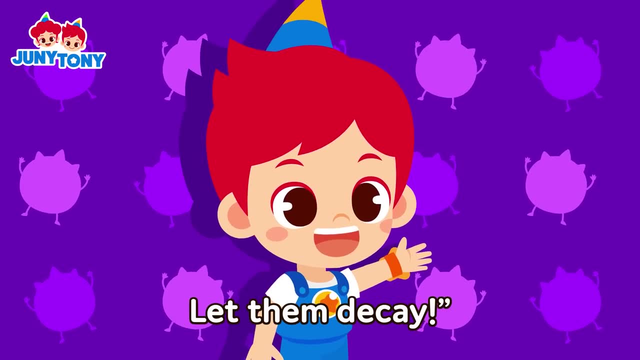 I'm Streptococcus Mutus the Great. I'm Streptococcus Mutus the Great. Hee, hee, hee, hee, I'll conquer your teeth. Rock'em away, Let them decay. Ha, ha, ha, ha, ha, ha. 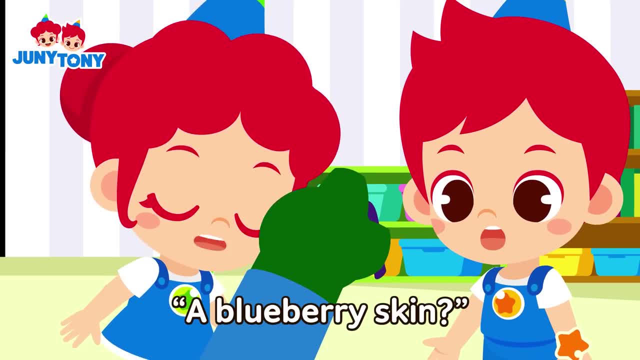 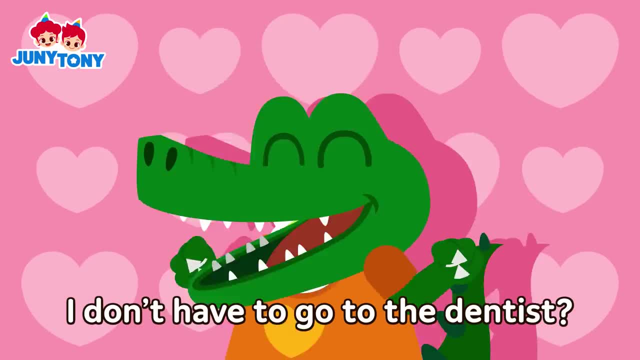 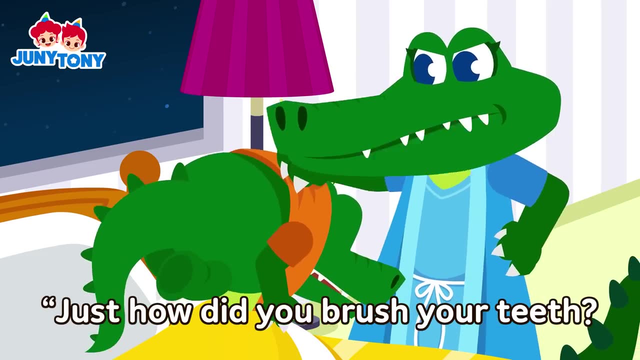 Oh, It's A blueberry skin. It wasn't a cavity at all. R-really, I don't have to go to the dentist. I'm so happy. Ha, ha, ha, ha, ha ha. Just how did you brush your teeth? 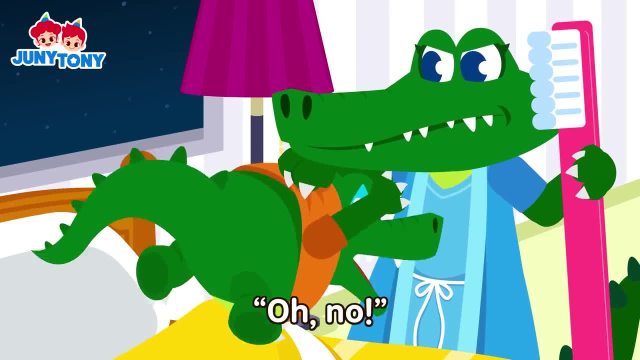 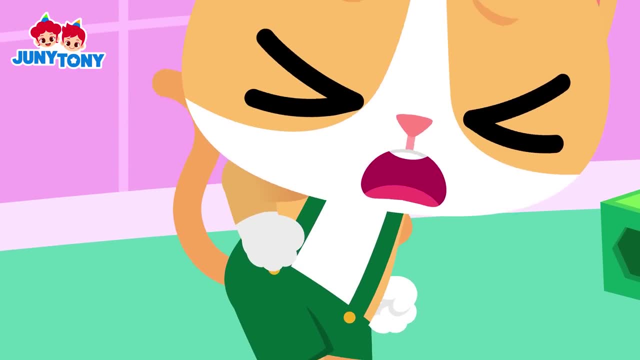 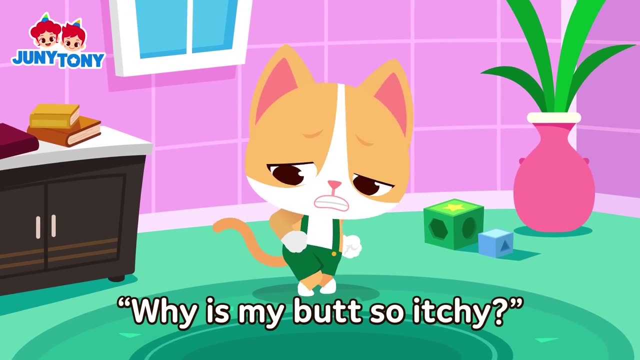 Come on, Let's brush again. Oh, No, Ha, ha, ha, ha ha, Oh, Hee, hee, Oh, Oh, Oh. Why is my butt so itchy? Oh, Oh, Oh, Oh, No, No. 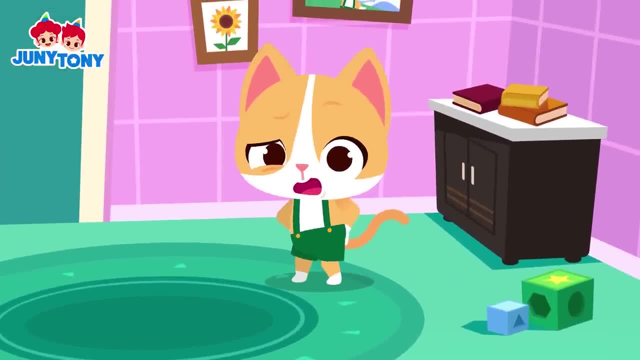 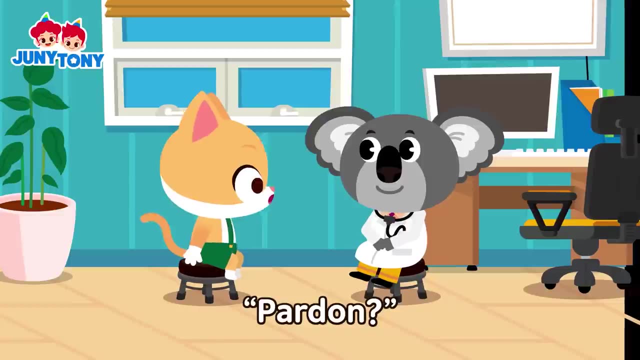 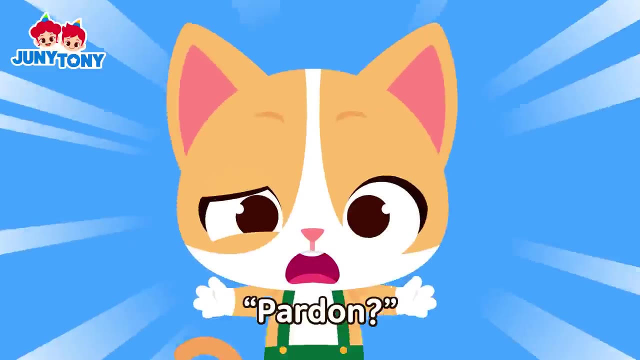 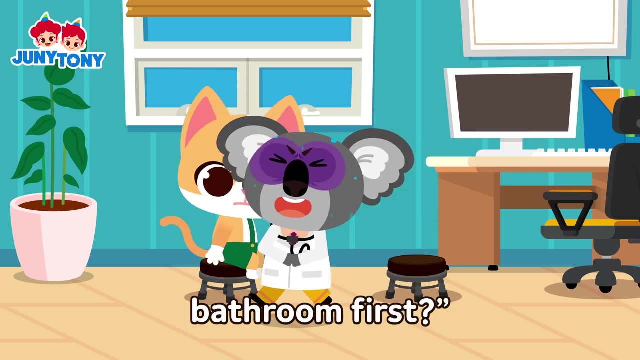 No, Guys, Ah, Oh Wait, Ah, Ah, It's because of the parasites, Pardon, It's okay, It happens. Parasites lay eggs on the butt, Pardon, May, May I go to the bathroom first? 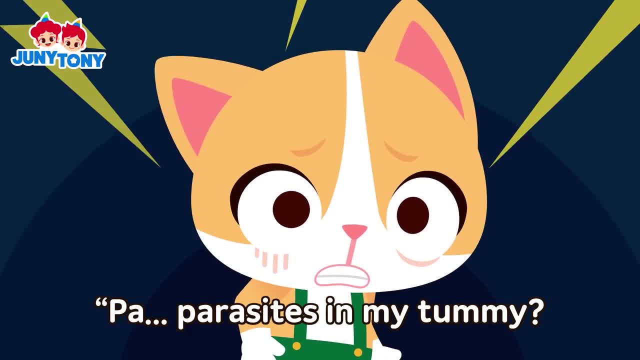 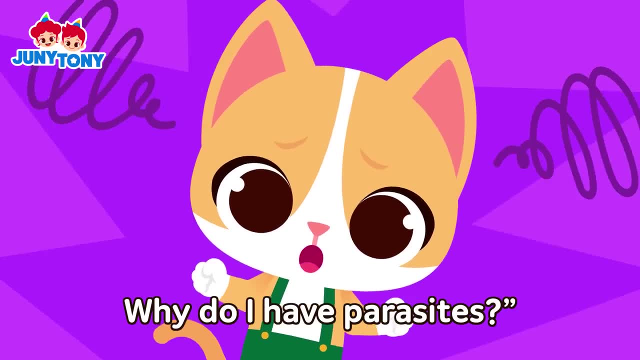 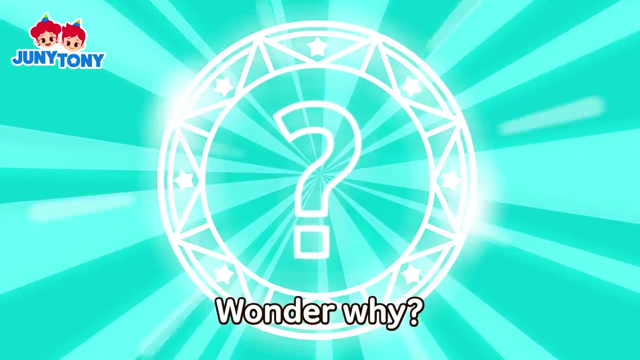 Parasites in my tummy, Laid eggs on my butt. Ah, Why do I have parasites? Juny Tony, Curious song: Choo choo, choo, choo, choo, choo, choo, Whir, Whir. 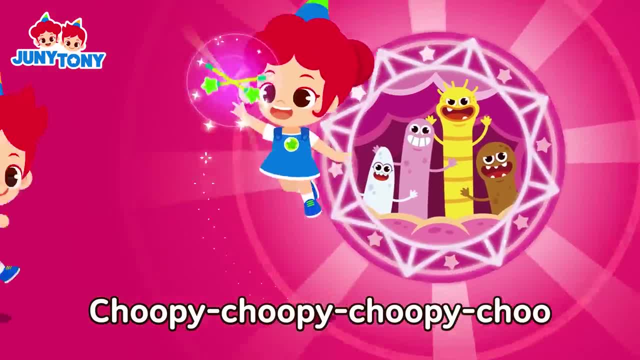 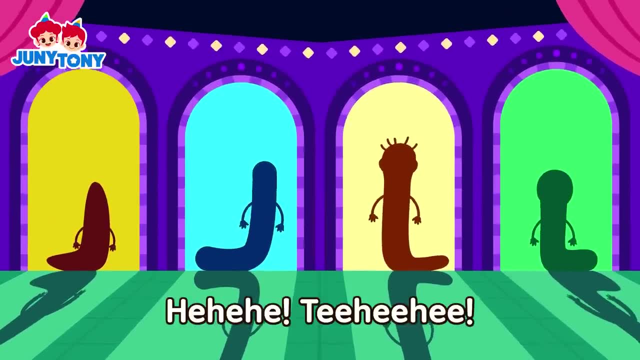 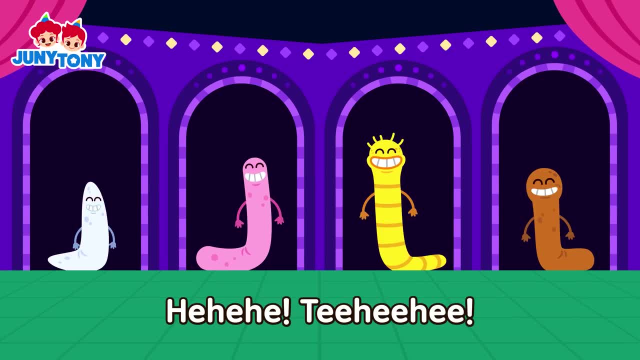 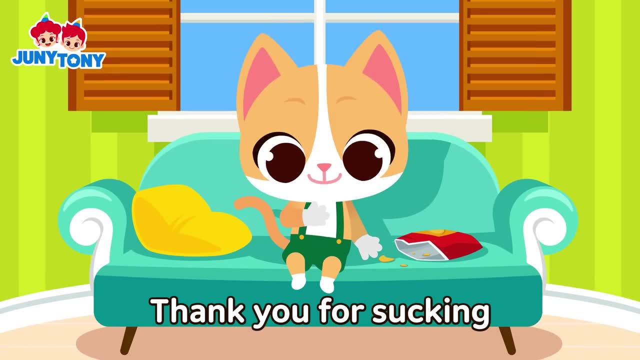 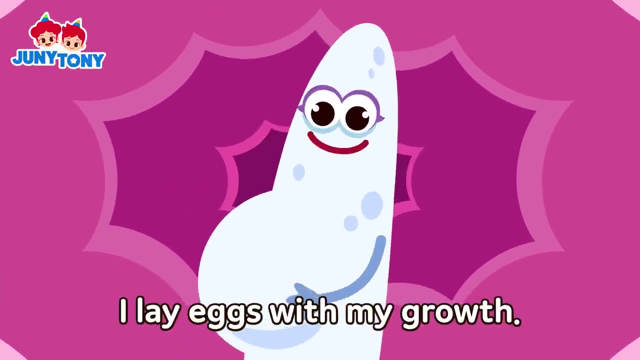 I'm Thread Worm. I'm Round Worm. I'm Tape Worm. I'm Huck Worm. I am Thread Worm. I came in through your mouth. Thank you for sucking your unwashed fingers right? I am Thread Worm. I lay eggs with my growth. 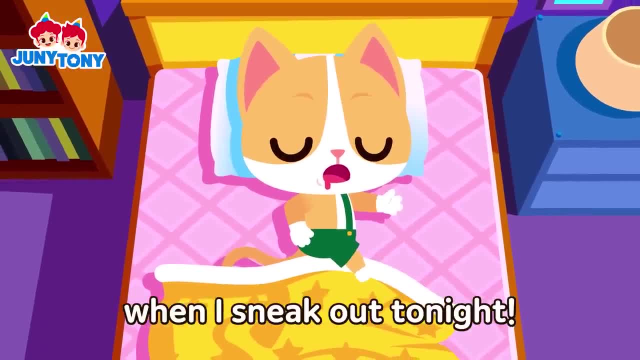 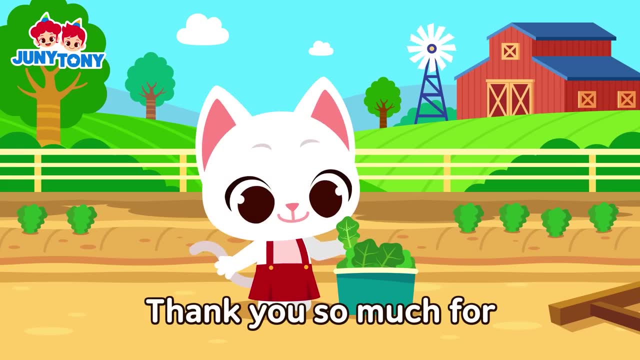 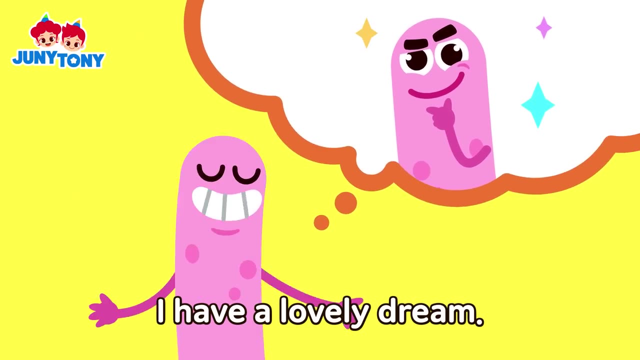 I'll lay eggs on your butt when I sneak out tonight. I am Round Worm. I came in through your mouth. Thank you so much for eating unwashed veggies. I am Round Worm. I have a lovely dream: I'll meet my partner and make a family of many. 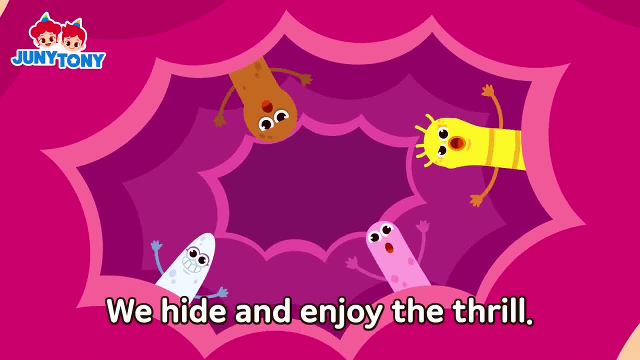 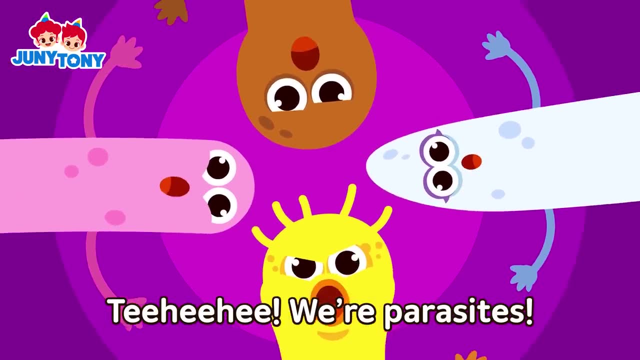 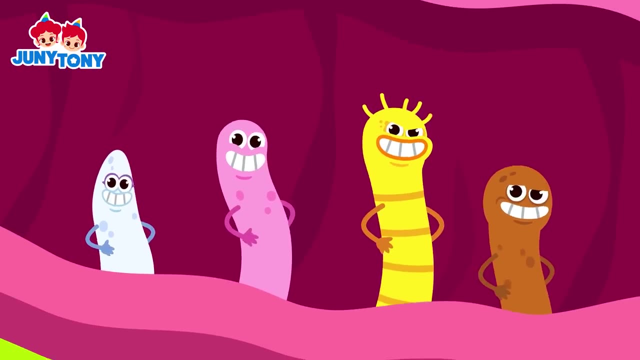 Take me where parasites we hide and enjoy the thrill. Steal nutrients. let's make a fuss. Take me where parasites we promise will stay still. Please don't get rid of us. Take me where parasites we hide and enjoy the thrill. I am Tape Worm. 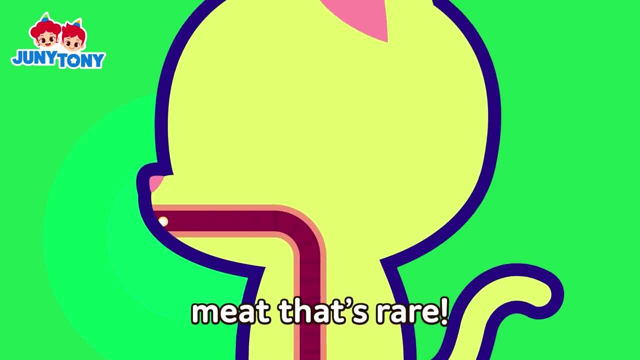 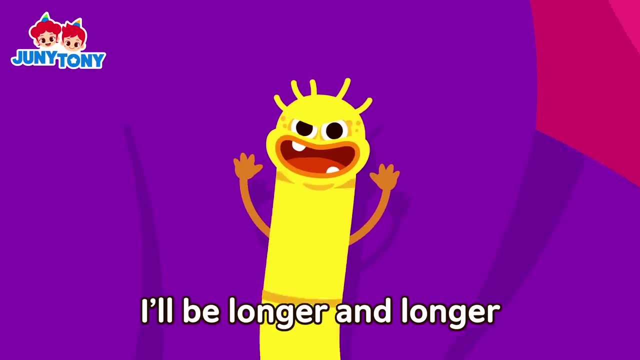 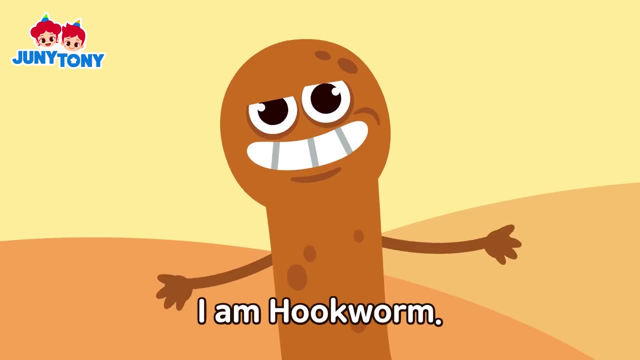 I came in through your mouth. Thank you for eating meat. that's rare. I am Tape Worm. I'm longer than you think. I'll be longer and longer than give you a stomachache. I swear I am Huck Worm. I came in through your skin. 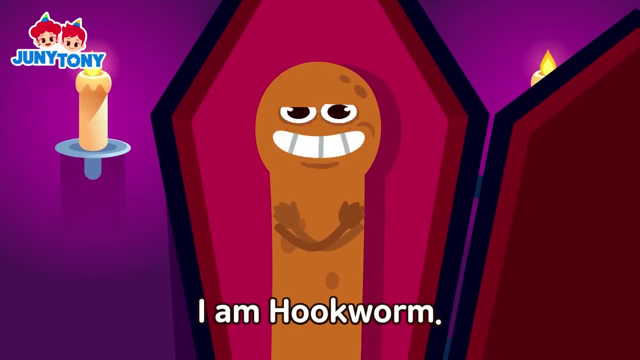 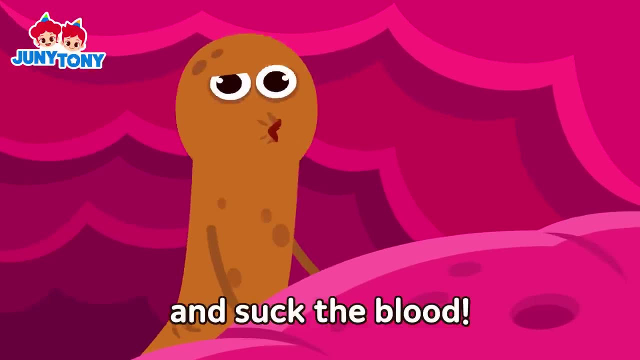 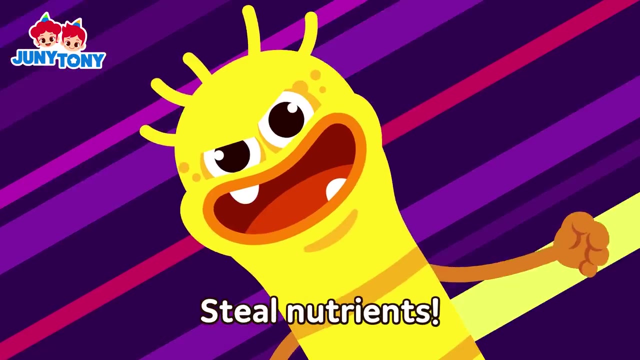 Thank you for playing in. I'm clean sand and mud. I am Huck Worm. I'm a vampire parasite. I bite the walls of the small intestine and suck the blood. Take me where parasites we hide and enjoy the thrill. Steal nutrients. let's make a fuss. 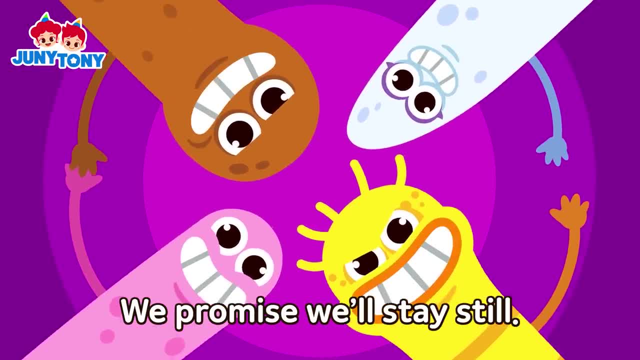 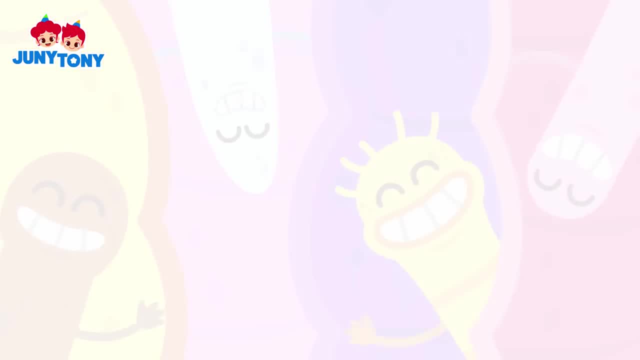 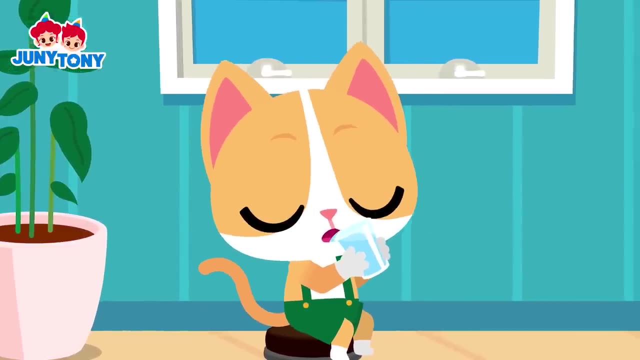 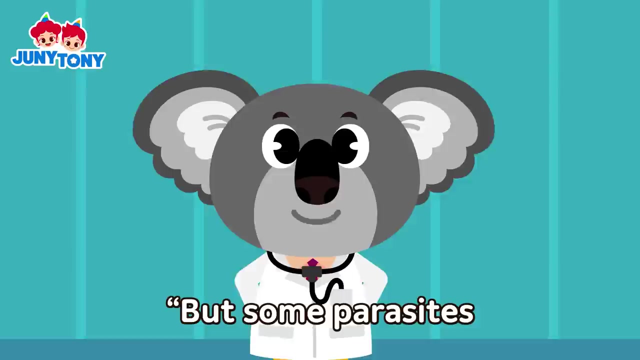 Take me where parasites we promise will stay still. Please don't get rid of us Here. take some pills. Thank you, Mmmm. Hmm, Nasty parasites Go away, Shoo shoo. But some parasites do strengthen your immunity. 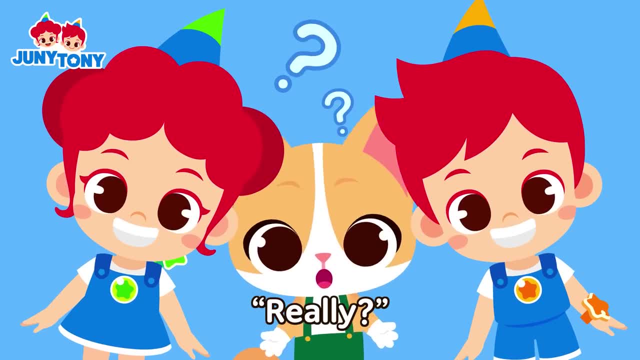 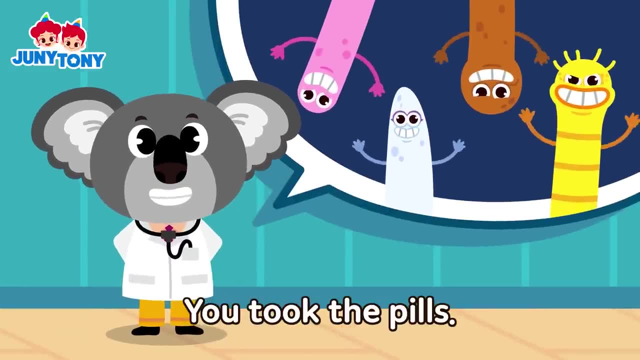 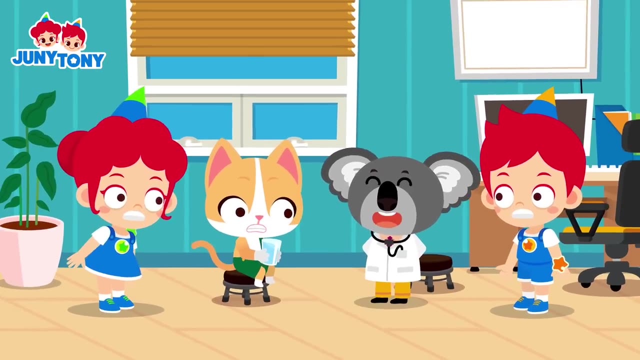 And even get rid of cancer cells- Really Uh-huh. But of course they are bad for your health, Don't worry. You took many, You guys. the pills, The parasites will come out in your pool. What Ah? 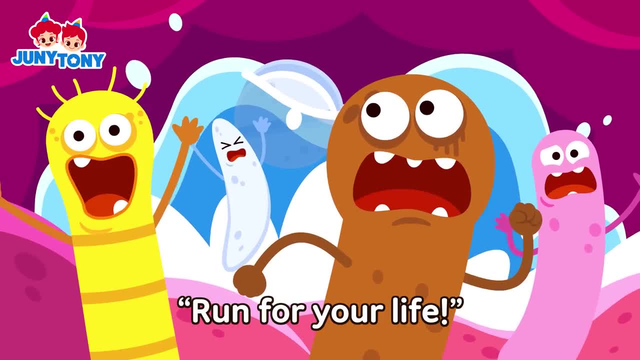 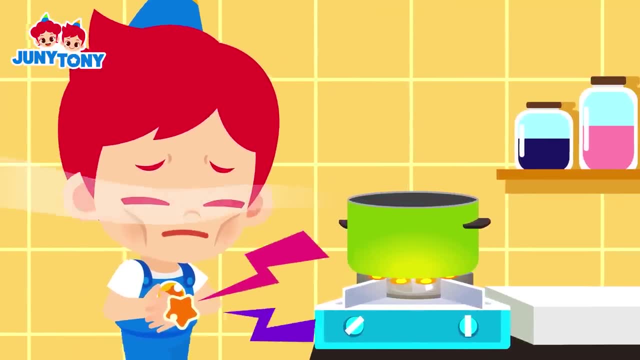 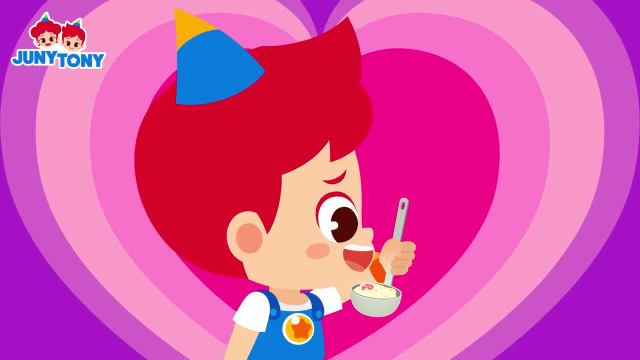 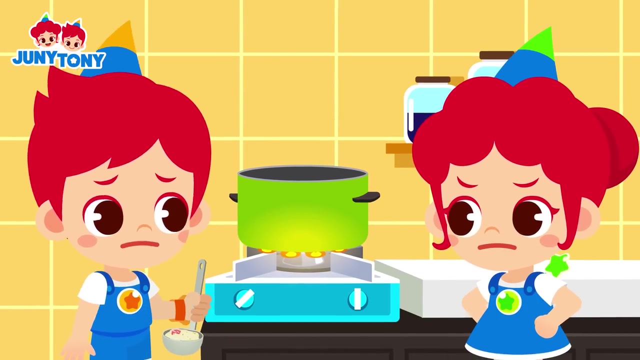 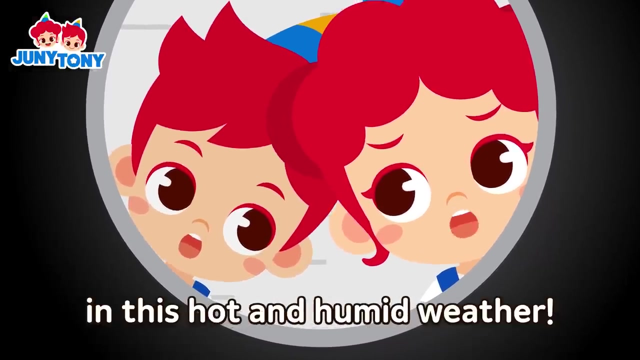 Atomatics Ready for your life? No, Tony, I know you're hungry, but it's not fully cooked yet. Come on, It should be good enough by now. It's really dangerous to eat uncooked food in this hot and humid weather. Look. 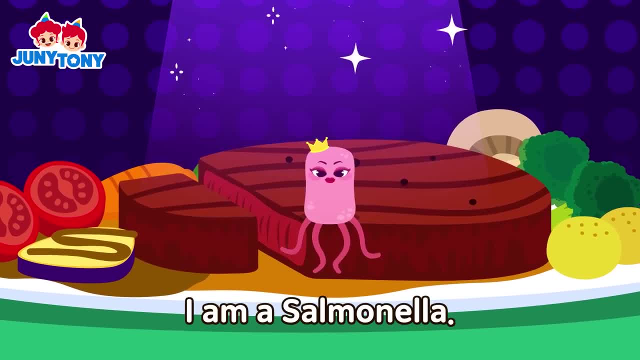 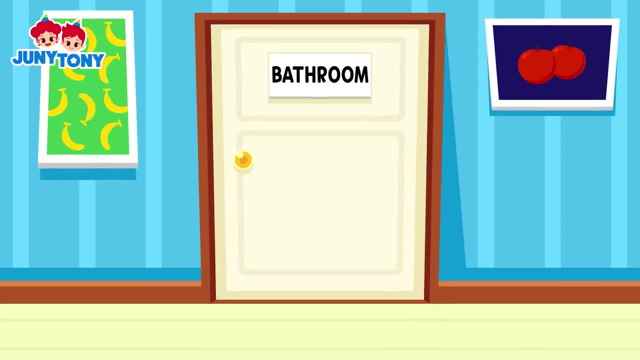 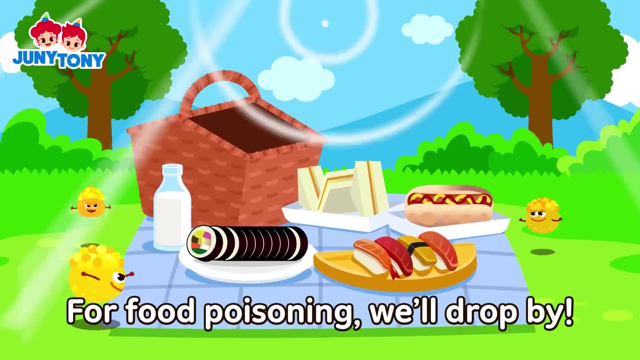 Hello, Have we met before- I'm a salmonella, Don't be afraid- fellas, The queen of food poisoning. Oh, poor thing, Meow Staphylococci. Poor food poisoning will drop by Full toxins. we're so thrilled. 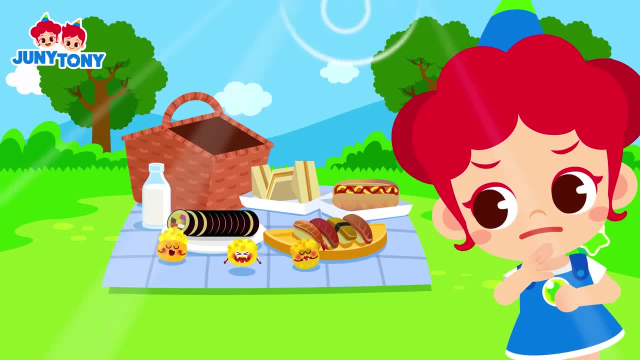 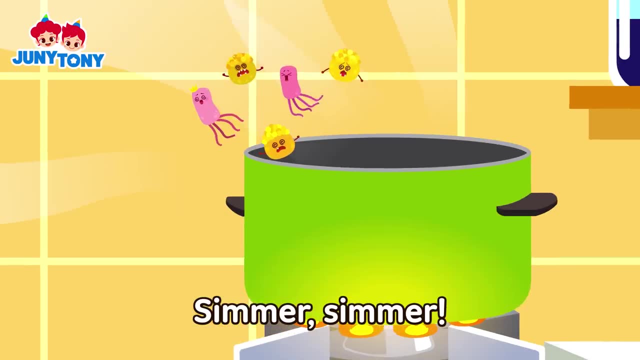 It's time to make them ill. No, no, you never will. Bubble washer hand snorrelly, sizzle sizzle. Cook your food early, Sipper, slipper all good, hot and slowly Remember. 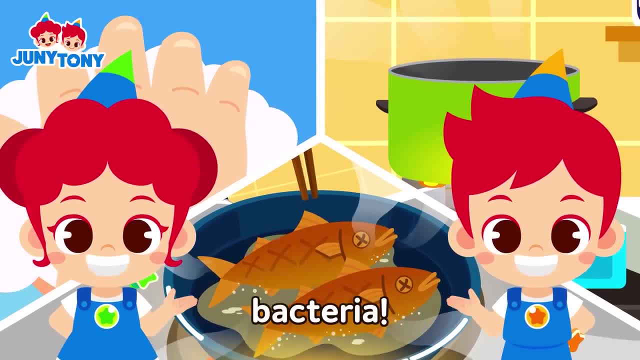 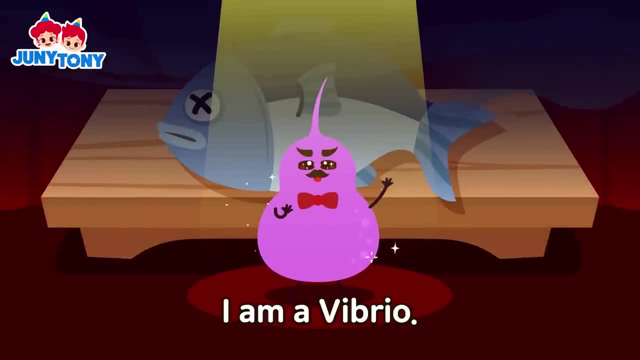 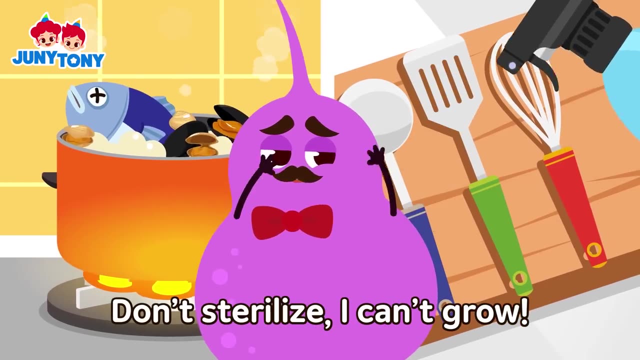 these three tips and you'll be safe from bacteria. I am also in this scenario. I am a Vibrio. I love seafood, so Please don't steam them. oh no, Don't sterilize. I can't grow, We're dangerous. 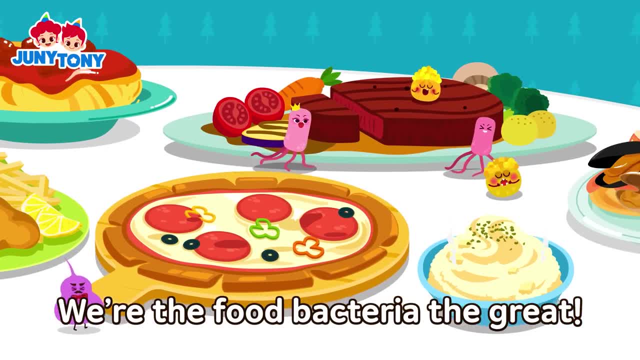 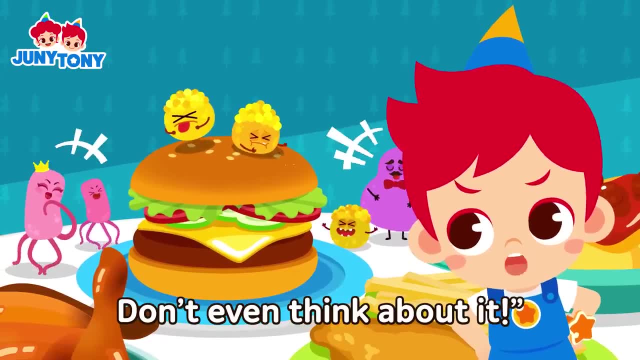 on your plate. We're the food bacteria of the great. Let's go make some trouble. My yibble-eeble-dabble-dabble-may Mean bacteria don't even think about it. Bubble washer hand snorrelly. 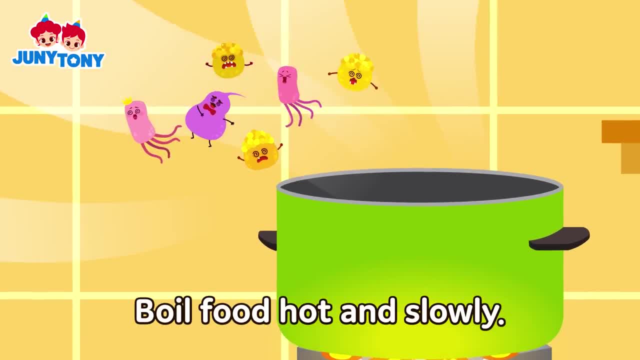 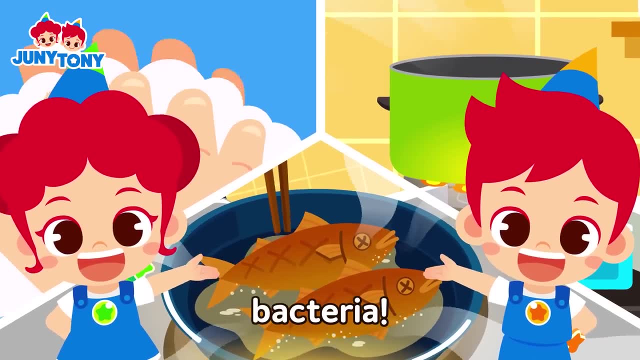 sizzle, sizzle, Cook your food early. Sipper slipper all good hot and slowly. Remember these three tips and you'll be safe from bacteria. Bubble washer hand snorrelly. sizzle, sizzle, Cook your food. 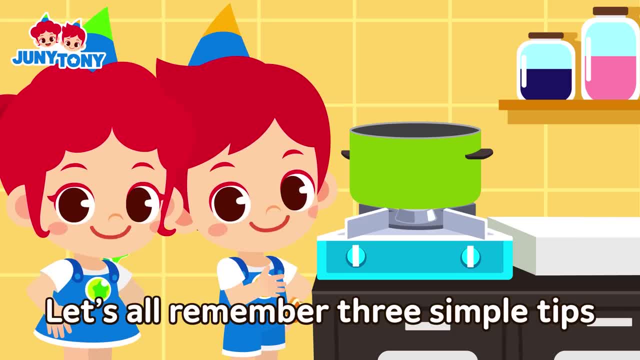 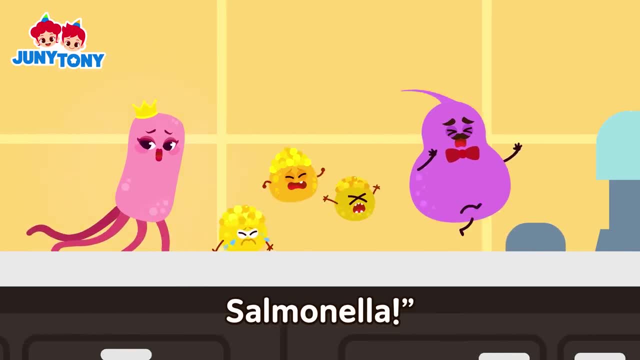 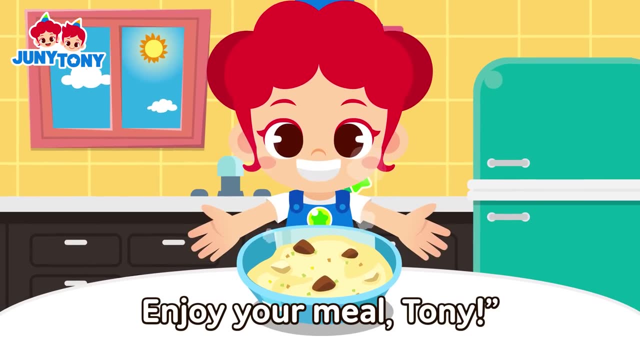 early Sipper slipper all good, hot and slowly. Let's all remember these three simple tips for our health. Boopsy, hup, wop, so vanilla Ta-da. Enjoy your meal, Tony Wow. 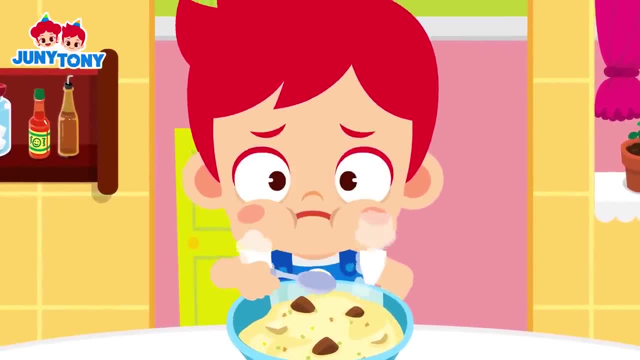 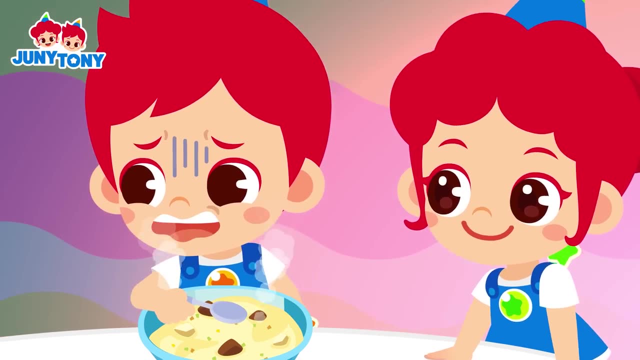 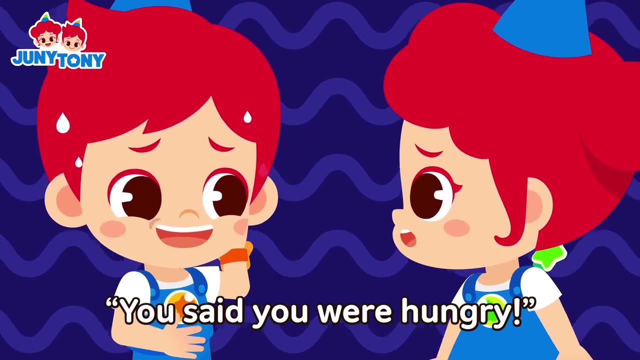 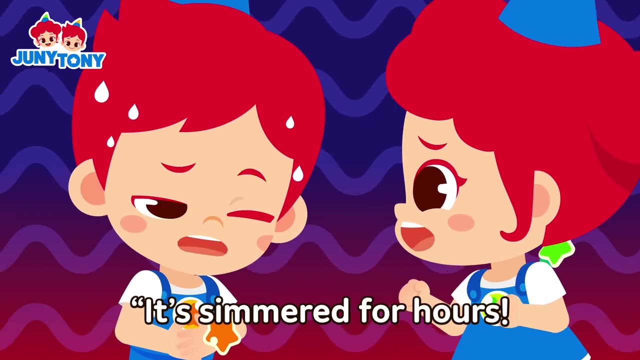 Now let me. It's yummy, Really. Have as much as you want. I think I'm full now. You said you were hungry. I think my tummy aches a little. It's simmered for hours. What are you? 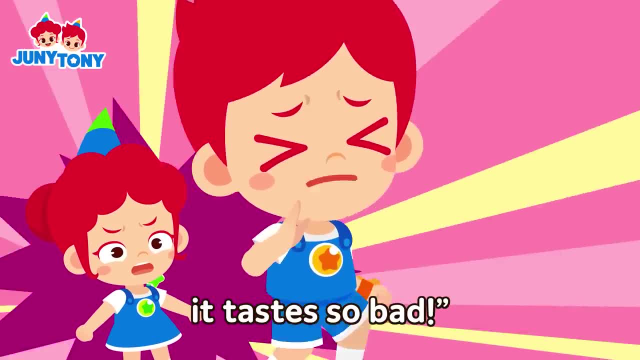 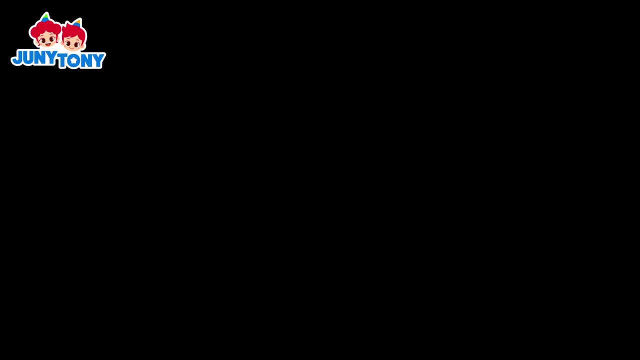 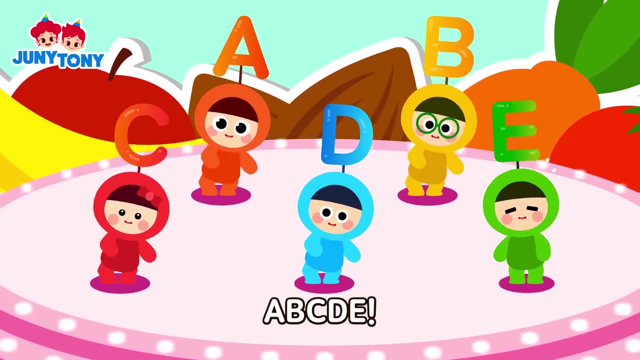 talking about. To be honest, it tastes so bad. Huh, What? What? Vitamin A, B, C, D, E, A, B, C, D, E, Vital, vital, vital, vital vitamin. It's the vitamin song. 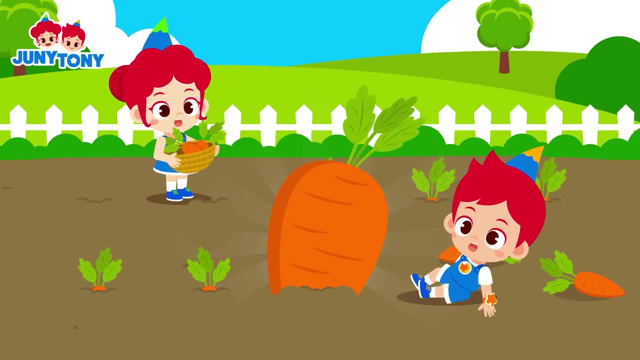 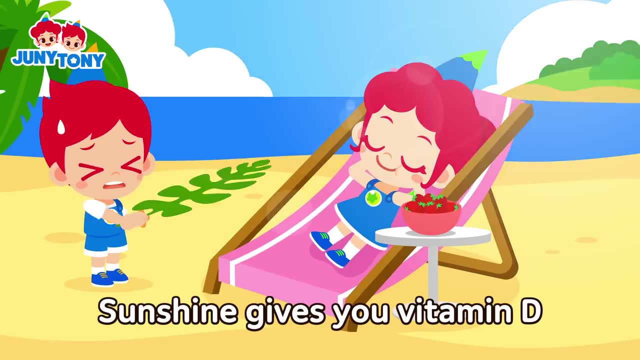 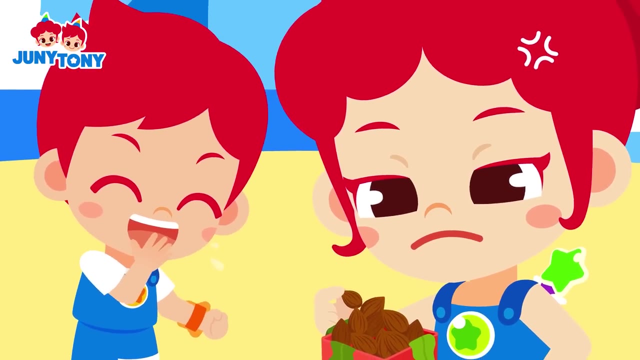 Carrot, carrot, vitamin A, A, Banana, banana, vitamin B, B, Strawberry, berry, vitamin C. sunshine gives you vitamin D, Almond, Diamond Almond, Vitamin E E, Vita, vita, vitamin A, B, C, D, E. 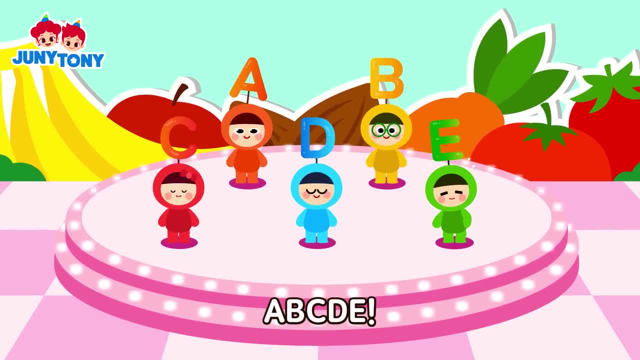 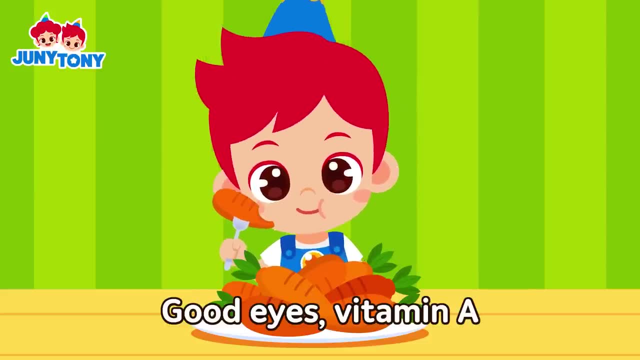 Vitamin A, B, C, D E. A, B, C, D E, Vita, vita, vital, vital vitamin, Good eyes. vitamin A A, Full of energy. vitamin B B: Go away fatigue. 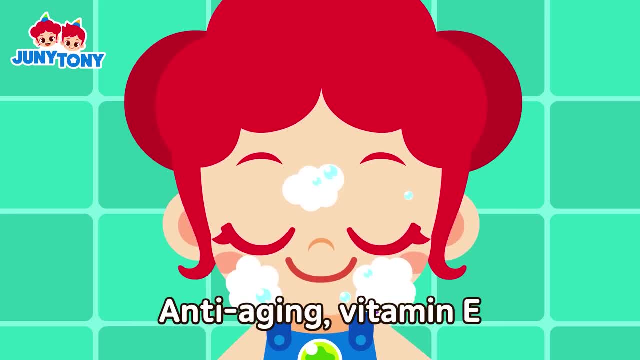 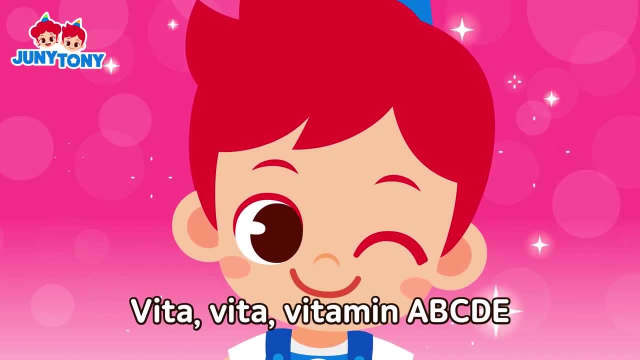 Vitamin C strong bones, vitamin D anti-aging, vitamin E, E Vita vita, vitamin A, B, C, D, E. Vitamin A, B, C, D E, A, B, C, D. 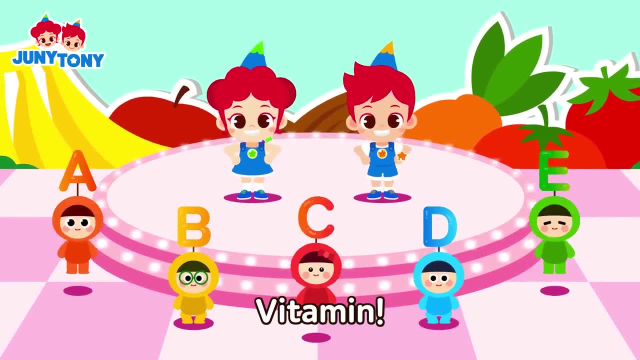 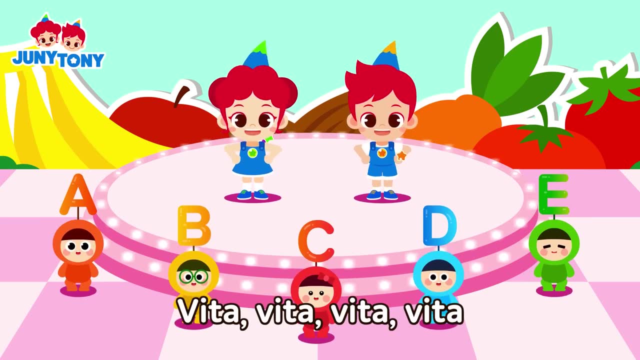 E. Vita vita, vital, vital vitamin. Grown taller. Vitamin A, B, C, D E. A, B, C, D E. Vita vita, vital, vital vitamin, Get prettier. 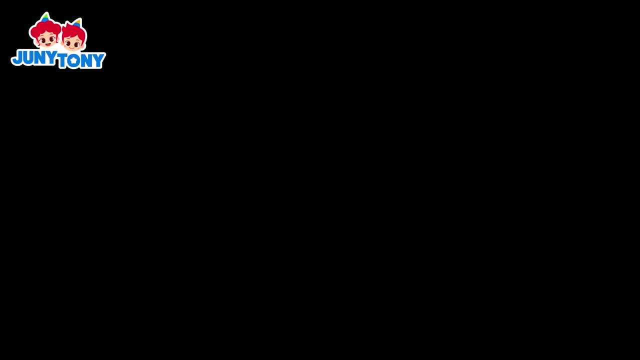 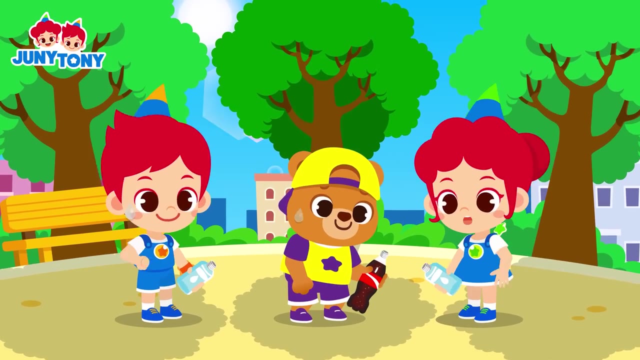 Vitamin A, vitamin B, C, D, E, D, E, A Glowing Kill the거든요 quelques décimos from a negativo dead weight: 麦다 xu 컵 59 han Heroin. 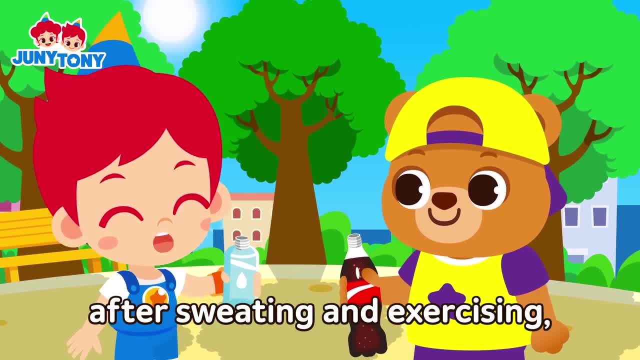 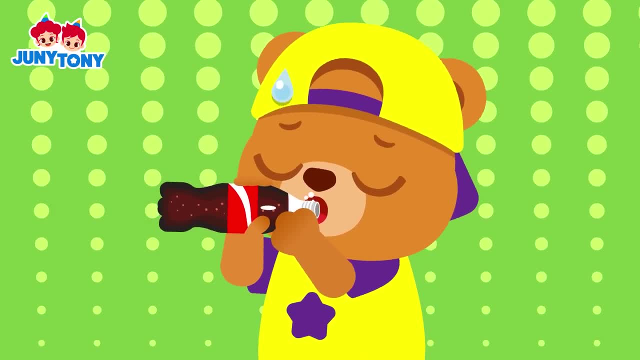 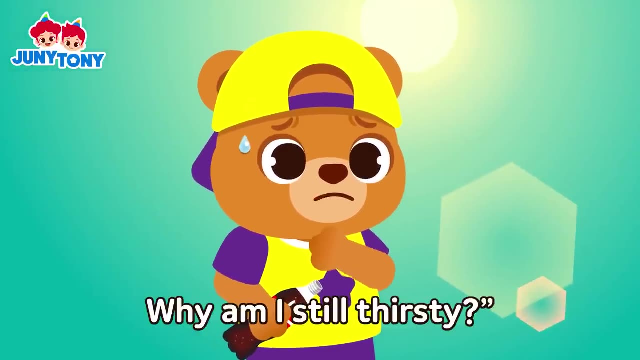 It sounds like from a nation where there are several esses or populations that need to turn the negative changes into rather beneficial sweat- desper Map회. There are also other elements related to aster. Sc Jacima. It's weird: I drank a soda. Why am I still thirsty? 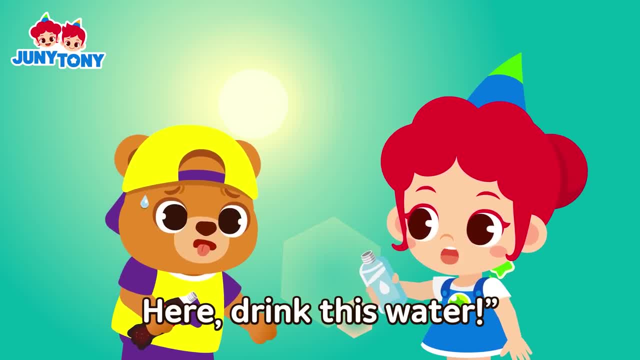 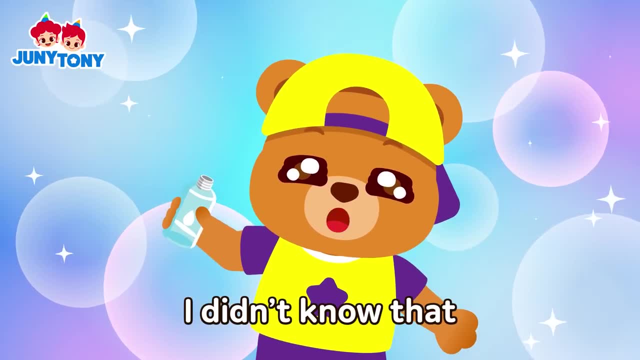 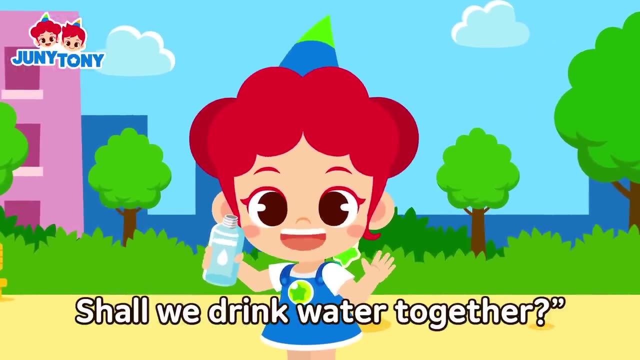 Beverages can't replace water Here. drink this water. Wow, It's so cool. I didn't know that water could be this good. You should drink water from time to time for your health. Shall we drink water together, Yeah? 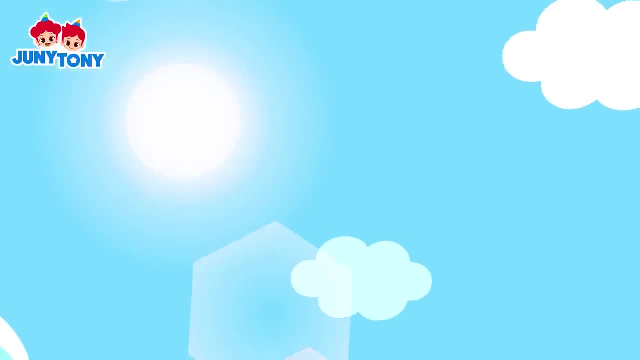 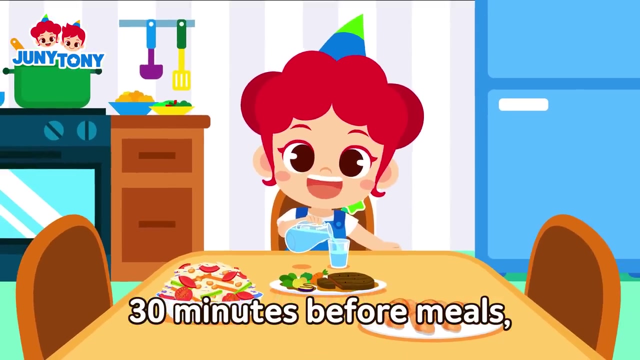 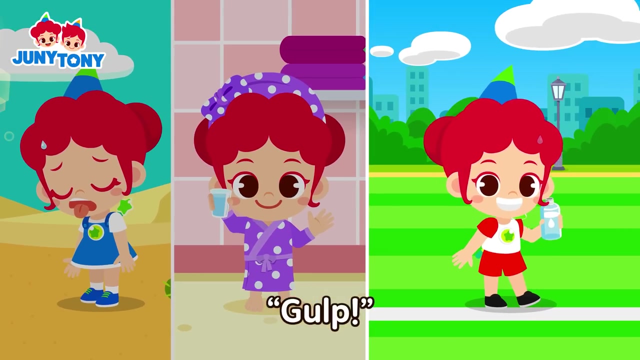 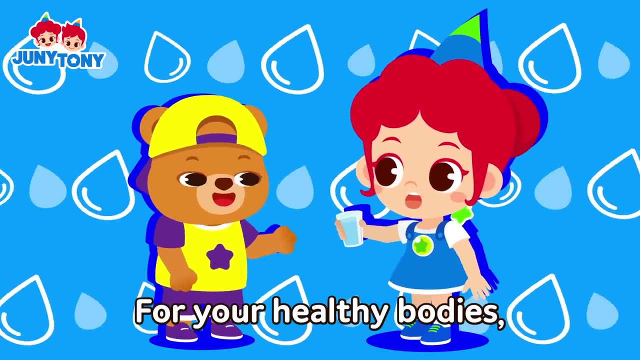 When you wake up in the morning, drink water 30 minutes before meals. drink water When you're thirsty, after shower, When you're sweaty, gulp, gulp, gulp. Sugary sweet beverages. oh no, no, never too much for your happy bodies. 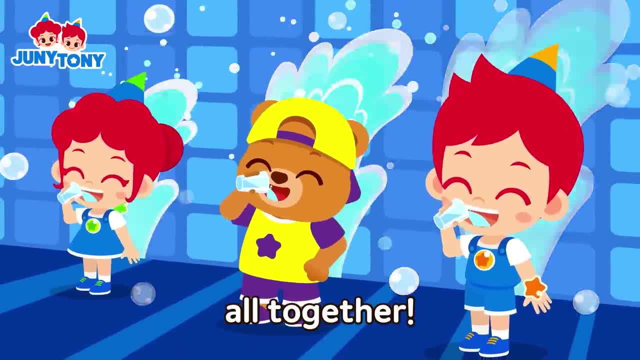 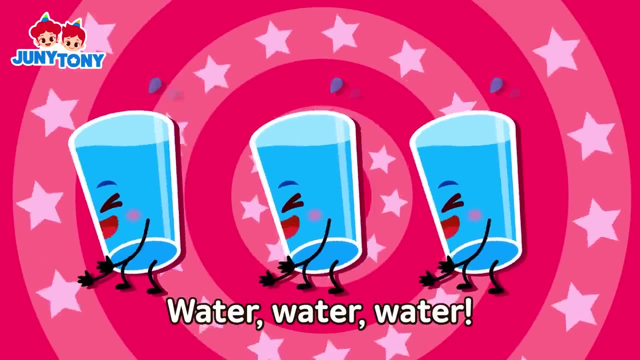 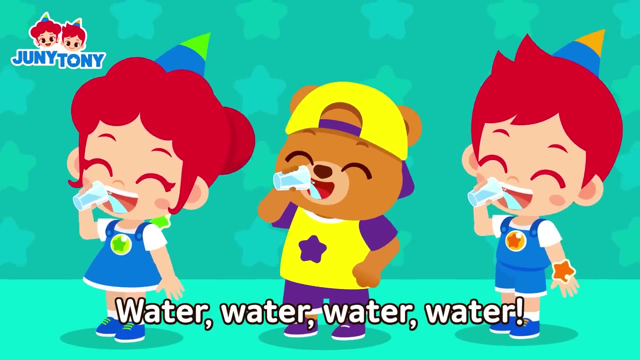 Let's drink water all together. Water, water, water. look at my glowing skin. Water, water, water. help me cool down. Water, water water. no waste in our bodies. Water, water, water, water. let's drink water together. 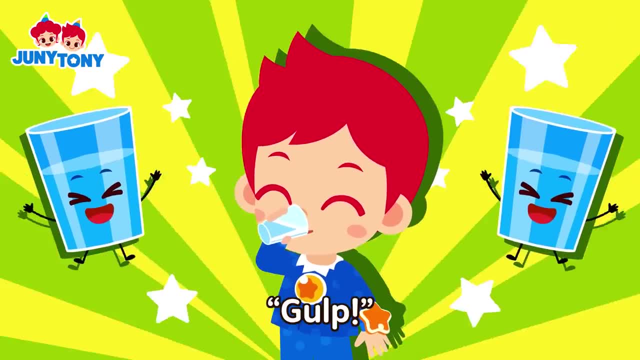 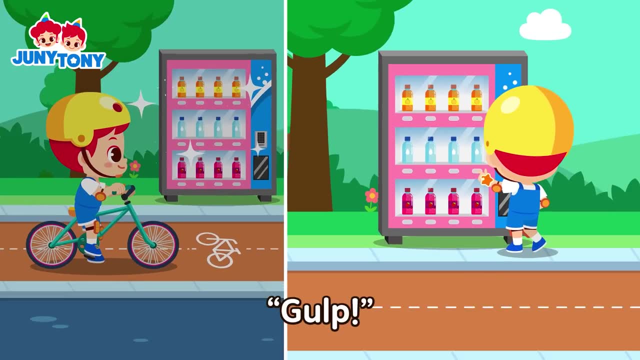 When you wake up in the morning, drink water. 30 minutes before meals, drink water. Drink slowly, drink thoroughly, drink frequently. 모르지 안 underneath 오물대의 들어갈 때 � Prett ganzeWow! Go go go, ha! 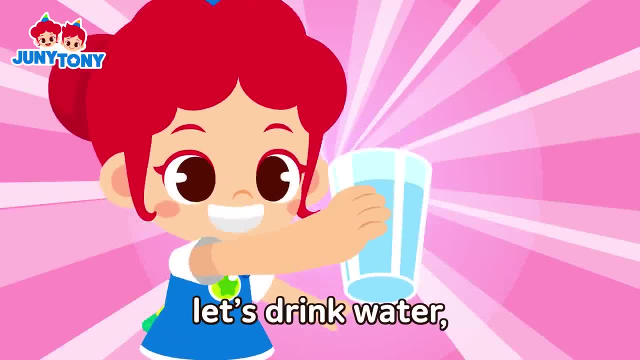 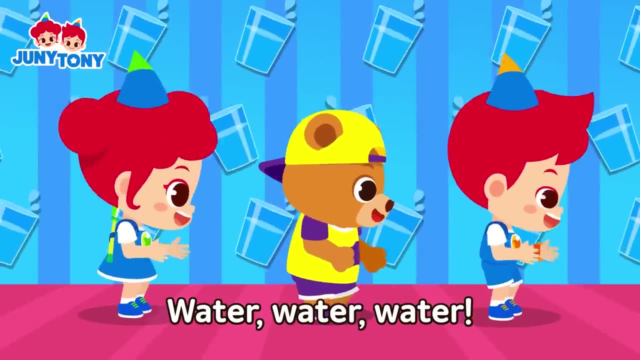 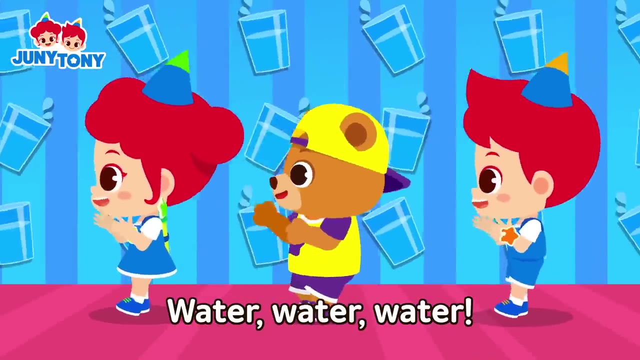 Sugary, sweet beverages, oh no, no, never too much for your happy bodies. Let's drink water all together. Water, water, water. Look at my glowing skin. Water, water, water. help me cool down. Water, water, water. No waste in our bodies. 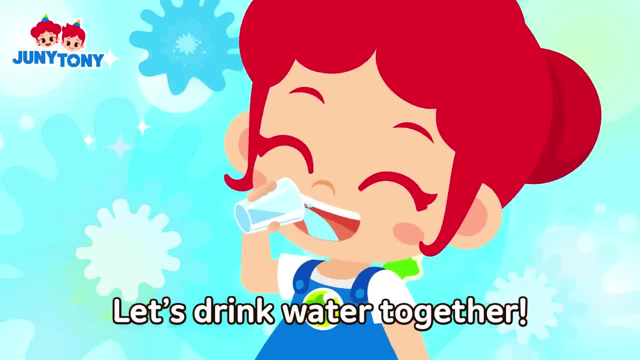 Water, water, water, water. Let's drink water together. Water, water, water, Water, water, water altogether. Let's drink water all together: Water, water, water. look at my glowing skin. Water, water, water. Look at my glowing skin. 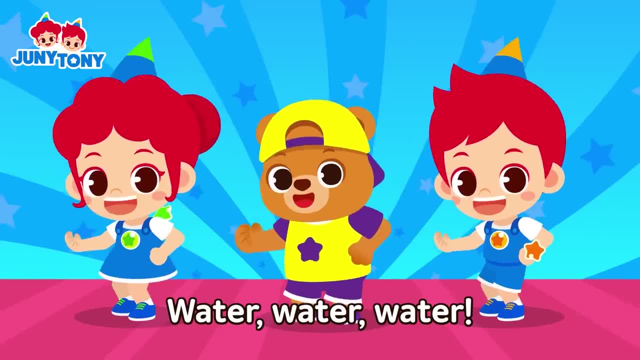 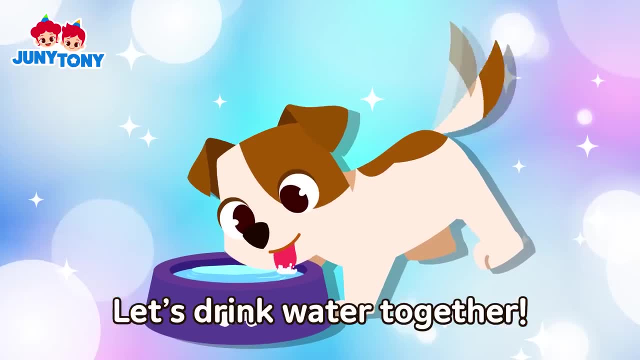 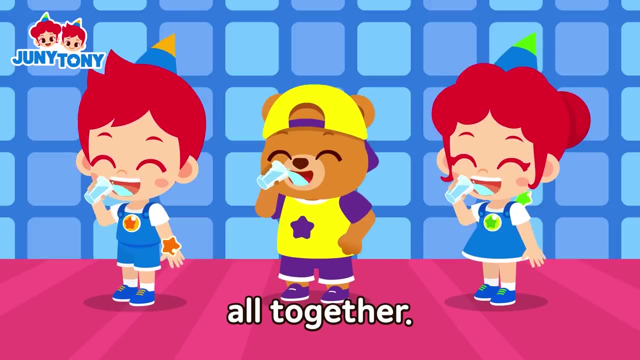 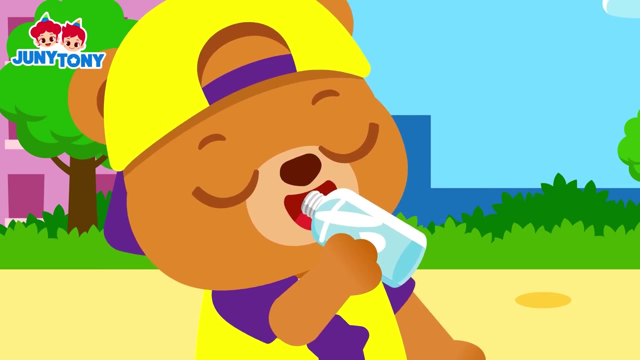 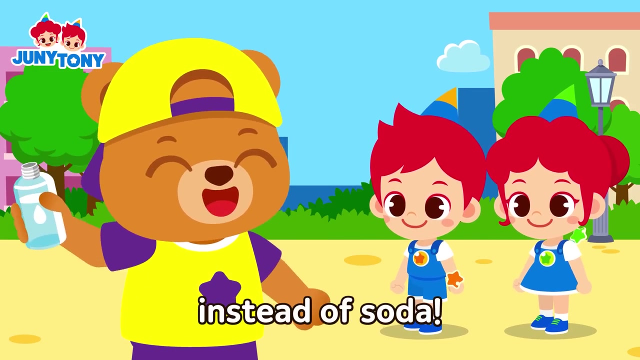 Water, water, water. Help me go to poop. Water, water, water. No waste in our bodies. Water, water, water, water. Let's drink water together For our happy bodies. Let's drink water All together. Wow, it's so cool. From now on, I'll drink healthy water instead of soda. 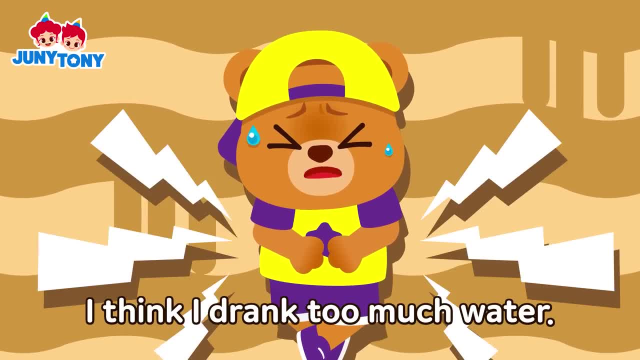 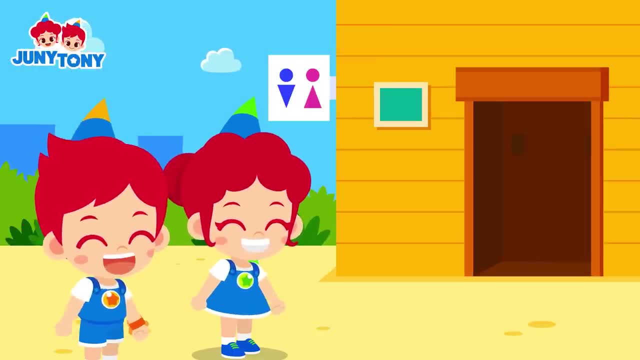 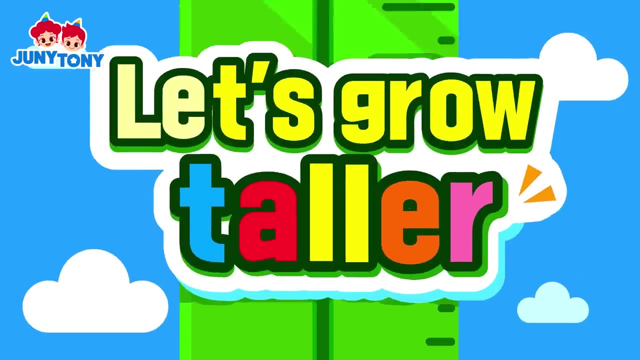 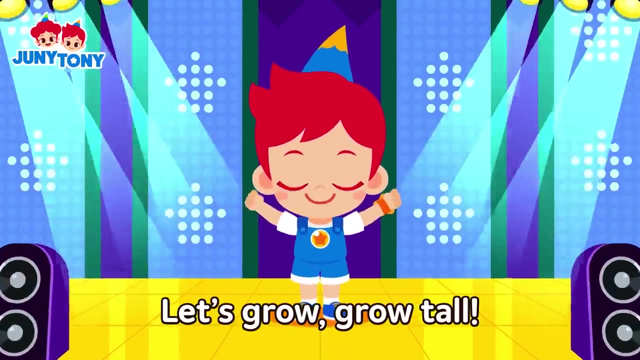 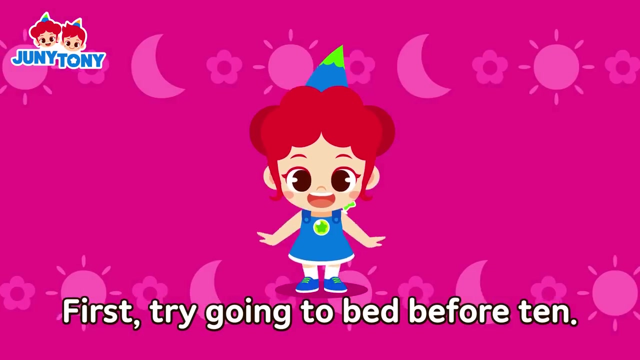 Oops, I think I drank too much water. I have to pee. Let's grow, grow taller. Let's grow, grow tall. Let's grow, grow taller. Let's grow, grow tall. Here are some tips on growing taller. First, try going to bed before ten. 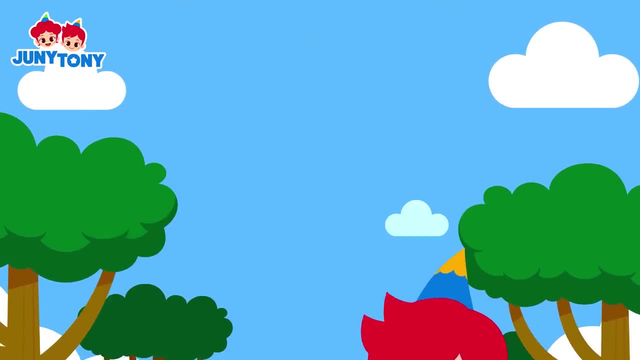 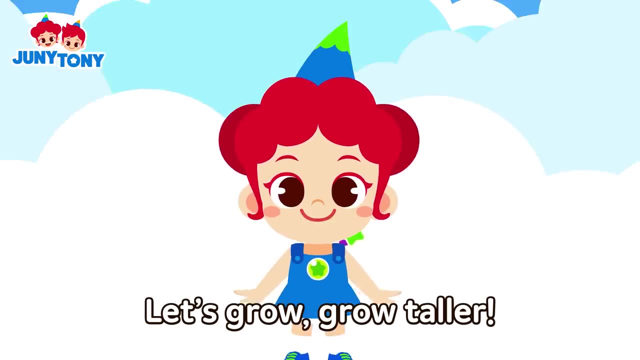 You can grow, grow taller then. Yes, that is right, going to bed before ten. You can grow, grow taller, then Let's grow, grow taller. Let's grow, grow tall. Sleep tight and wake up early. Let's grow, grow taller. Let's grow, grow taller. 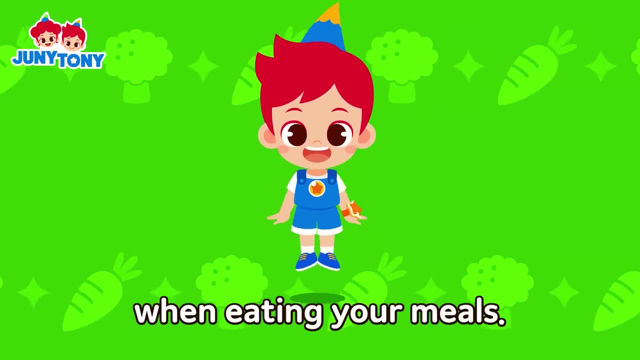 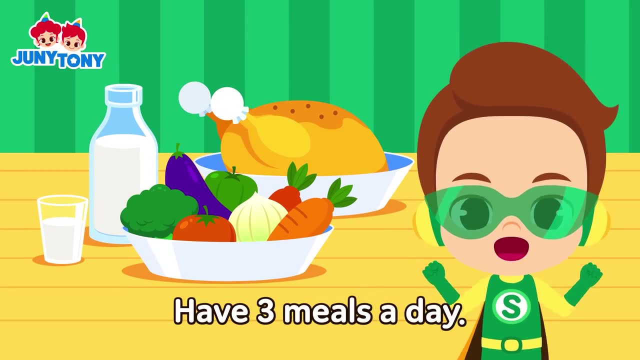 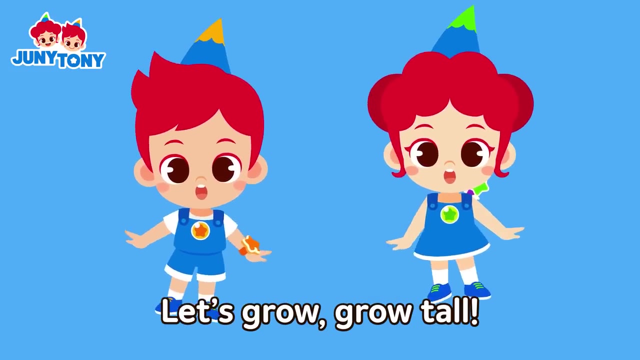 Never be picky when eating your meals. You can grow grow taller then. Yes, that is right, have three meals a day. You can grow, grow taller then. Let's grow, grow taller. Let's grow, grow tall. Don't be picky with food. 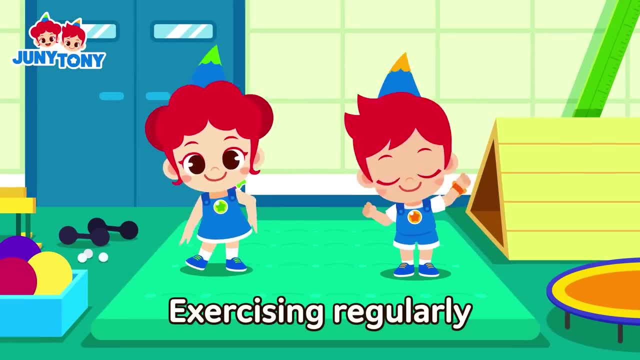 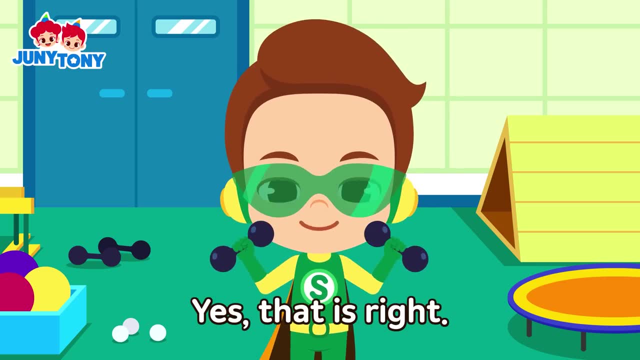 Let's grow grow tall. Exercising regularly makes you grow tall. You can grow grow taller then. Yes, that is right. going to bed before ten: You can grow grow taller then. Yes, that is right. have three meals a day. You can grow grow taller then. 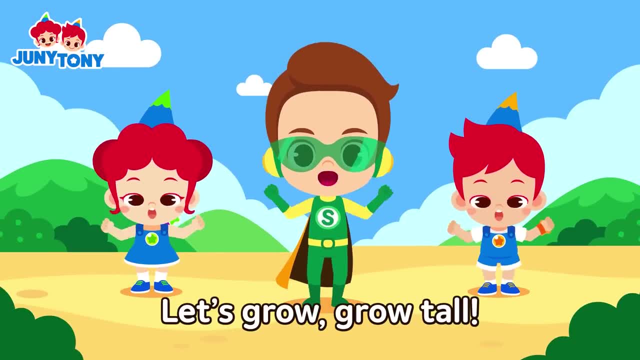 Yes, that is right. have three meals a day. You can grow, grow taller. then Let's grow, grow taller. Let's grow, grow tall, Exercising regularly. Let's grow, grow tall. Let's grow, grow taller. Let's grow, grow tall.